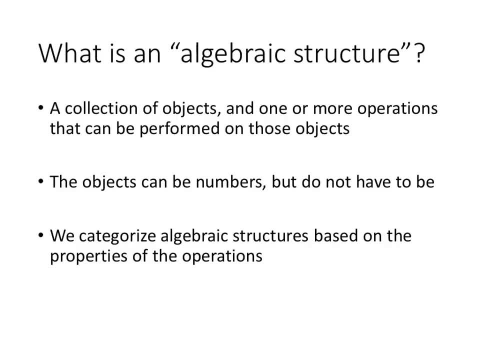 We could add them or multiply them or do something else, And we're going to categorize algebraic structures based on the properties of those operations, based on how many operations there are and what properties those operations have. Why do we care about doing this? Why do we want to categorize these algebraic structures? 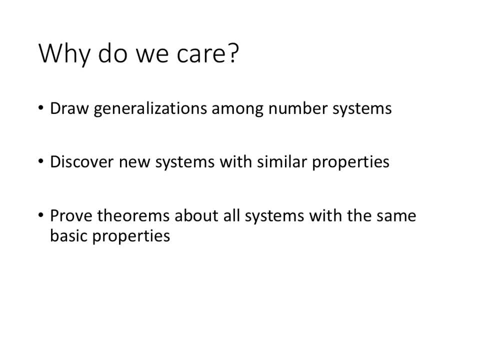 Well, there's a few reasons. One is that we can draw generalizations among number systems. So when we look out into the mathematical world and we see various different systems, including numbers and matrices and functions and all these other different things, 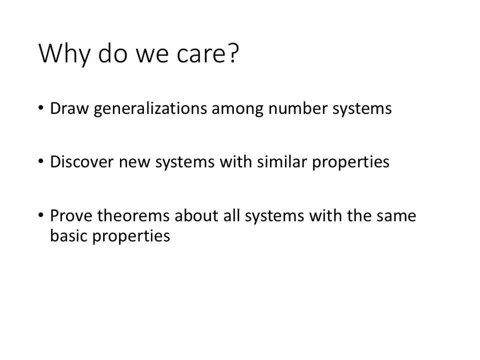 using algebraic structures, allows us to draw connections between those seemingly different systems. We can also, using this method, discover new systems that have similar properties to the ones that we're more familiar with. And finally, and this is probably the most important reason, 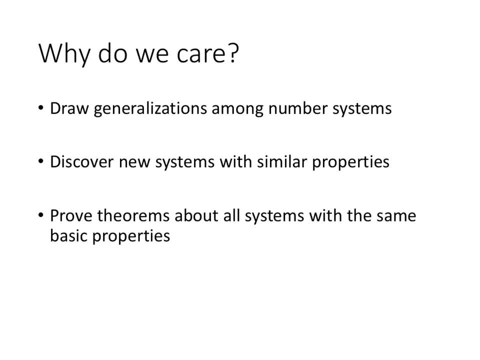 is that we can prove theorems about all systems with the same basic properties. So one of the systems we're going to talk about is groups. So once we know what a group is, if we prove a theorem about all groups, then that theorem applies to all groups that ever have been and ever will be. 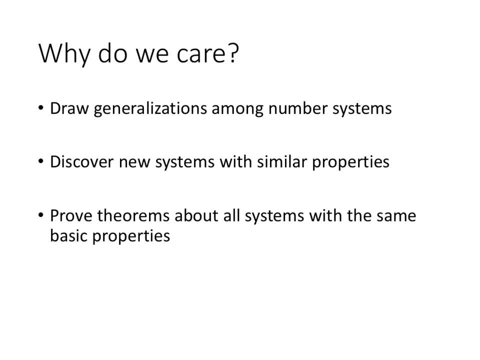 including groups that we haven't even discovered yet. We'll know things about those groups because we proved theorems about all groups. So that really is the main reason why we care about algebraic structures. So, speaking of groups, that's going to be the first type of algebraic structure we're going to talk about. 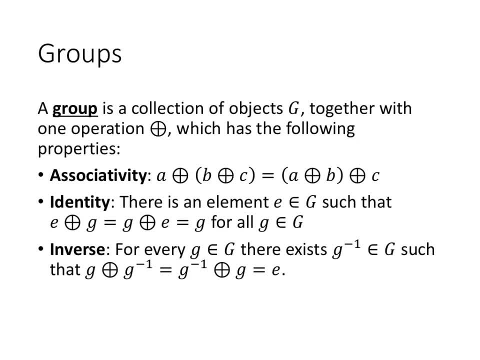 So I'm talking about these algebraic structures kind of in order from least complicated to most complicated, although you can kind of argue that It's really in the order of fewest properties to most properties. So the group is the simplest type of algebraic structure that we're going to talk about. 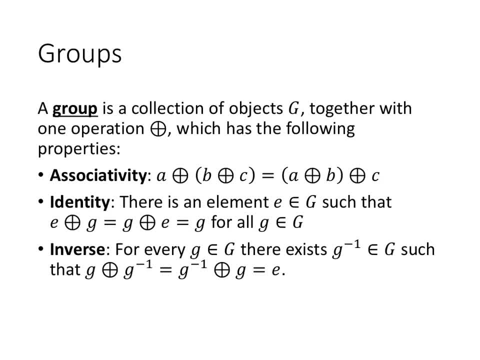 simply because we've got these objects, the set of objects that we're calling g. So g here is the set of objects, And then we've got our operation, which I'm calling this sort of plus in a circle, And I'm just intentionally using an unfamiliar symbol there just to indicate that this really could be any operation. 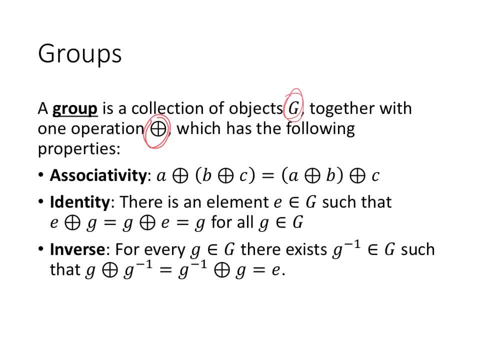 It could be addition, it could, but it could also be multiplication, It could be something else, So just some operation. we have to have a symbol for it. So I'm using this plus in a circle symbol, And then we've got three properties, and the three properties are associativity. 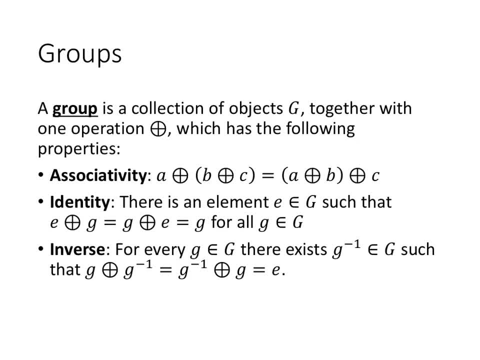 So I'm, talking about these algebraic structures kind of in order from least complicated to most complicated, although you can kind of argue that. 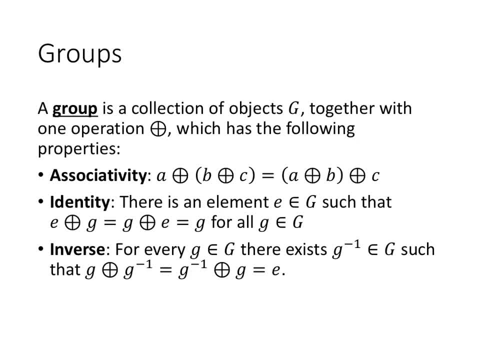 It's really in the order of fewest properties to most properties. 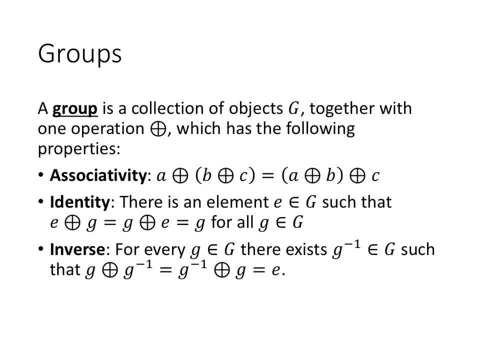 So the group is the simplest type of algebraic structure that we're going to talk about, simply because we've got these objects, the set of objects that we're calling g. So g here is the set of objects. 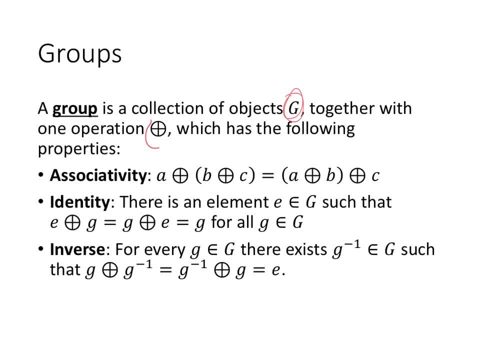 And then we've got our operation, which I'm calling this sort of plus in a, circle. 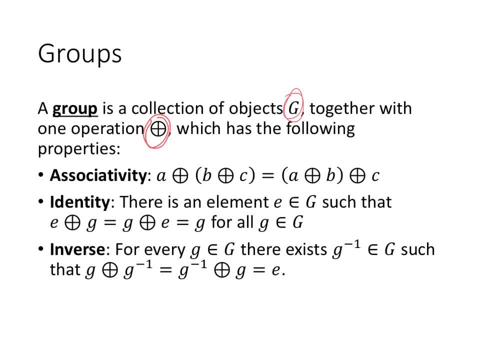 And I'm just intentionally using an unfamiliar symbol there just to indicate that this really could be any operation. It could be addition, it could, but it could also be multiplication. It could be something else. 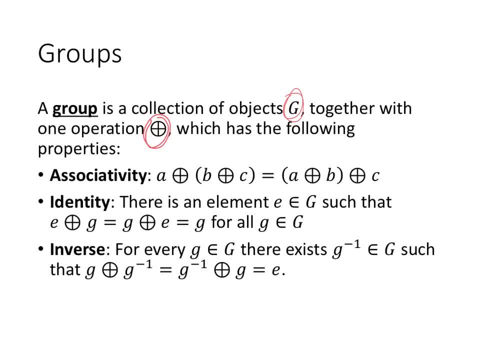 So just some operation, we have to have a symbol for it. So I'm using this plus in a circle symbol. 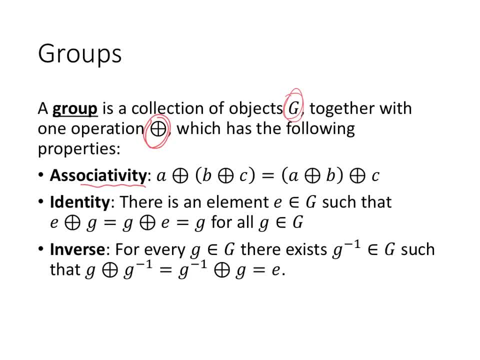 And then we've got three properties and the three properties are associativity. 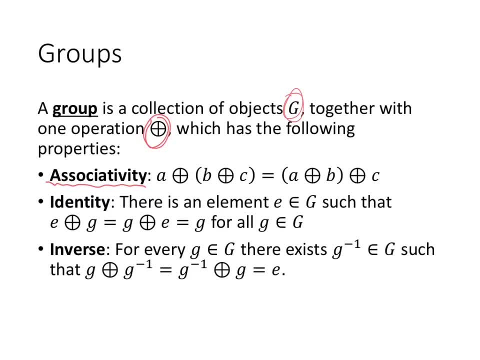 And that means that if I have three of these objects, the way that I group those objects doesn't matter. So if I have three objects that I want to use, this operation on if I do the second one in the third one together and then tack on the first one, that's the same as if I do the first two together and then tack on the third one. 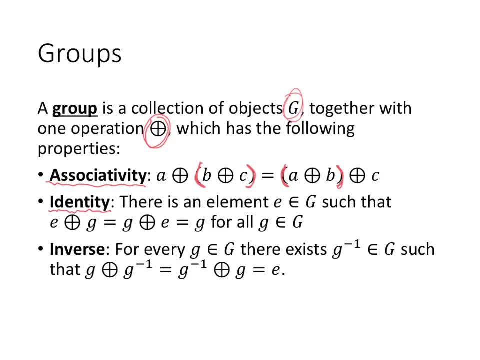 The next property is identity. So that means that there's a special element that we'll call e, although again, that's just sort of a general term. So in practice, this element might be called zero. It might be called one. So it's just some element of this group so that when I use that operation on with my, identity element, nothing happens. 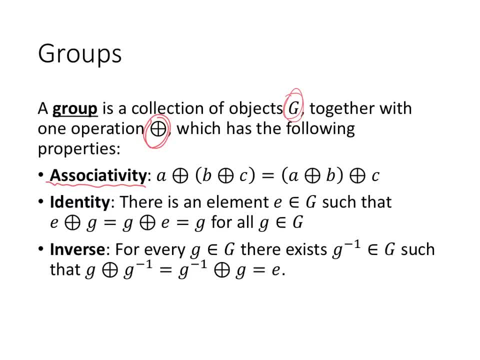 And that means that if I have three of these objects, the way that I group those objects doesn't matter. So if I have three objects that I want to use this operation on, if I do the second one in the third one together and then tack on the first one. 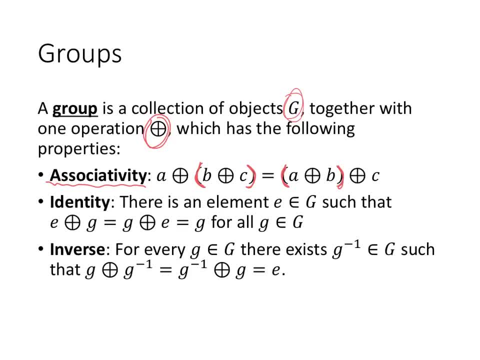 that's the same as if I do the first two together and then tack on the third one. The next property is identity, So that means that there's a special element that we'll call e, although again that's just sort of a general term. 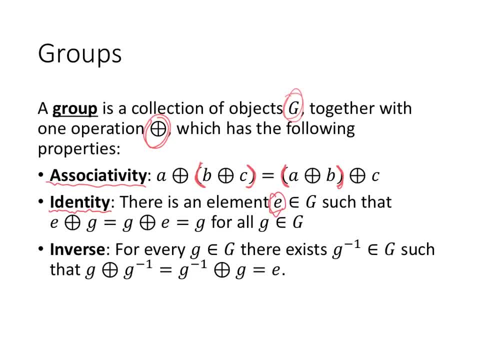 So in practice this element might be called zero, It might be called one, So it's just some element of this group, so that when I use that operation on with my identity element, nothing happens. So e plus g is the same as g plus e, and that just gives me g back. 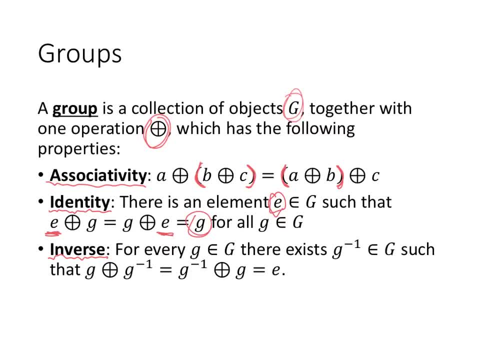 And then, finally, the third property is inverse. So that means that for every element of this group there's an inverse element, which we often write g to the minus one. But again, depending on what this group actually is, we might have a notation for it that's different than that. 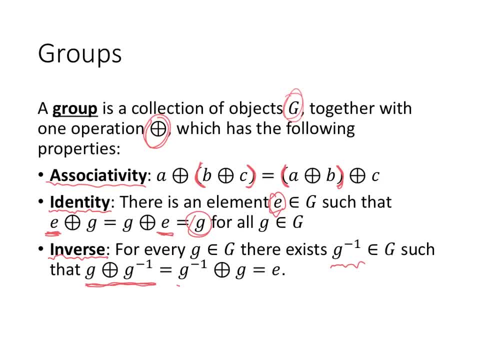 But when we do our operation with g and its inverse in either order, we just get back the identity Again. Okay, so this is all very abstract. Let's talk about some examples. Okay, so there's lots of examples of groups. 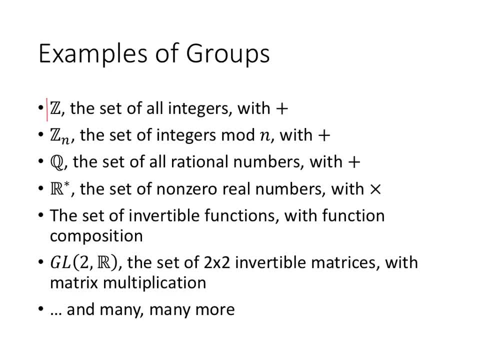 So let's start with probably the simplest example, which is the set of integers. Now, I'm using notation here: This bold-faced z just represents the set of all integers, That's whole numbers, positive, negative and zero, And the operation we're using is just a regular old addition. And so to verify that this is a group, 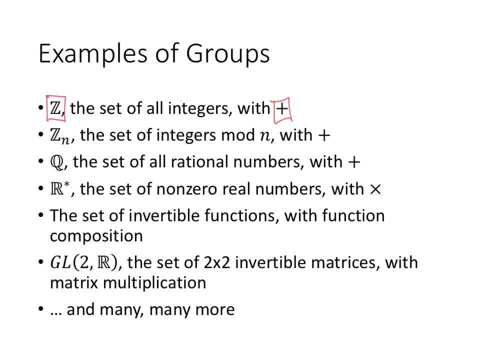 there's three things that we need to check. We need to check that addition is associative, which means we need to know that for any integers- a, b and c, a plus b plus c- should be the same as a plus b plus c, and that's a property that we know about integers. 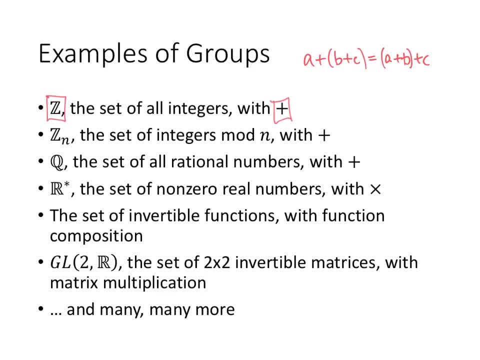 We also need to make sure that there's an identity. In this case, the identity for integers is zero, because a plus zero is equal to zero plus a, which is equal to a. Notice that I'm not calling it e, like I did on the previous slide, because in this case, 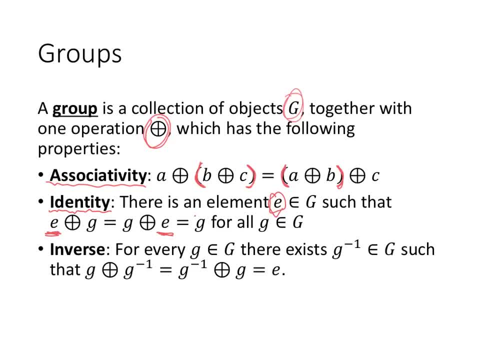 So e plus g is the same as g plus e and that just gives me g back. And then finally, the third property is inverse. So that means that for every element of this group, there's an inverse element, which we often write g to the minus one. But again, depending on what this group actually is, we might have a notation for it that's different than that. But when we do our operation with g and its inverse in either order, we just get back the identity. Again. 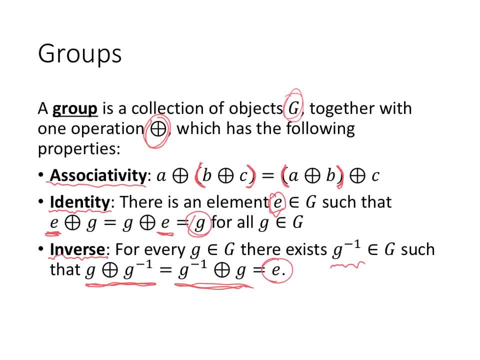 Okay, so this is all very abstract. Let's talk about some examples. Okay, so there's lots of examples of groups. 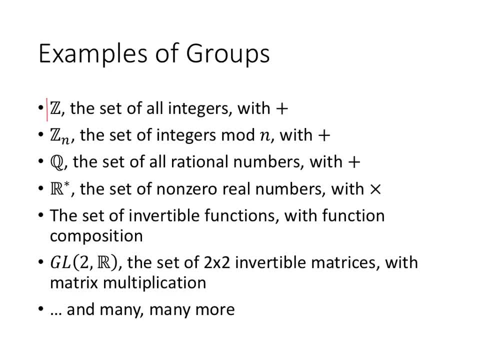 So let's start with probably the simplest example, which is the set of integers. Now, I'm using notation here. This bold-faced z 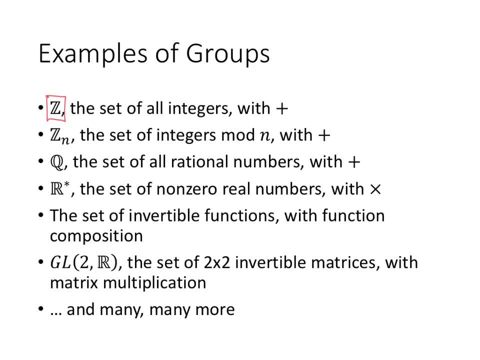 just represents the set of all integers. That's whole numbers, positive, negative, and zero. 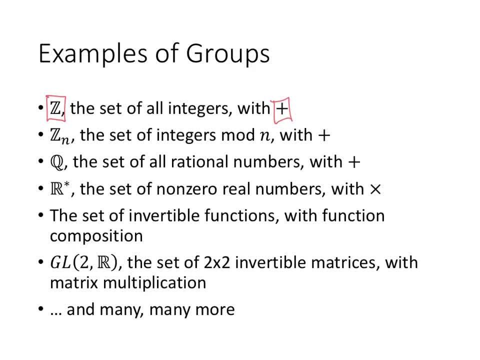 And the operation we're using is just a regular old addition. And so to verify that this is a group, there's three things that we need to check. We need to check that addition is associative, which means we need to know that for any integers a, b, and c, a plus b plus c should be the same as a plus b plus c, and that's a property that we know about integers. We also need to make sure that there's an identity. In this case, the identity for integers is zero, because a plus zero is equal to zero plus a, which is equal to a. 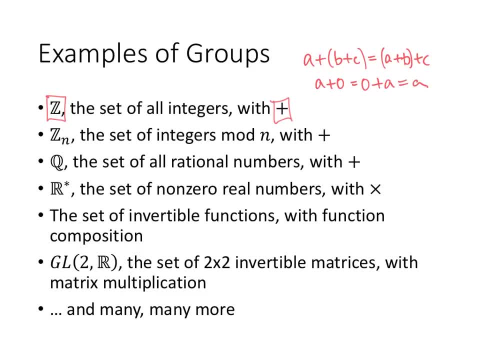 Notice that I'm not calling it e like I did on the previous slide, because in this case, we know what that identity is. We know that identity is a good old zero. 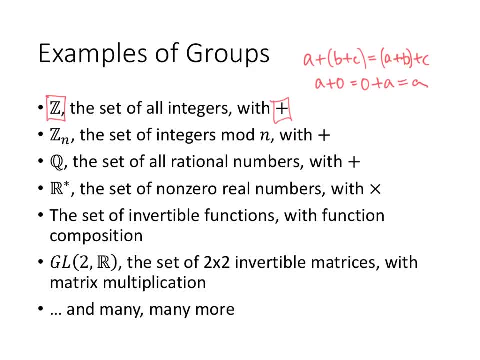 Finally, we have a requirement that we have to have an inverse for every integer. And in this case, for every integer a, the inverse of a is actually negative a, because negative a plus a gives us back that identity, which is zero. 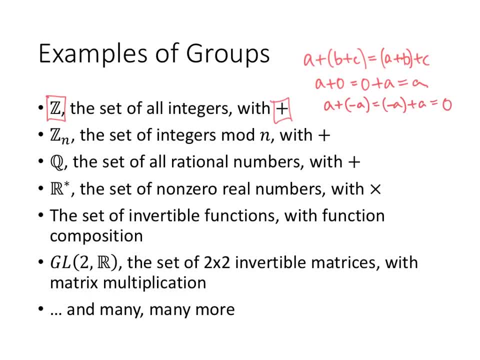 So again, I'm not calling it a to the minus one, because in this case, we specifically know that if I have any integer a, the additive inverse of that integer a is negative a. 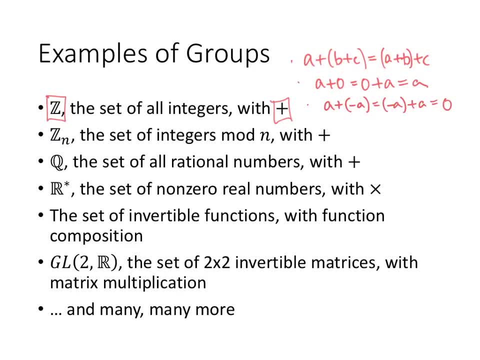 So those three lines there tell me that this is group. So I'm not going to go through and check all the properties for all of these examples, but that's the idea. That's what you would have to do to verify that 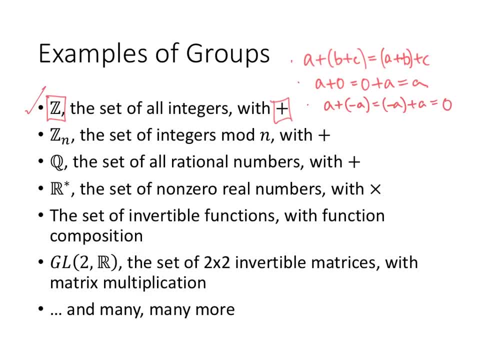 these things really are groups. So just going down the line here, the next example is set of 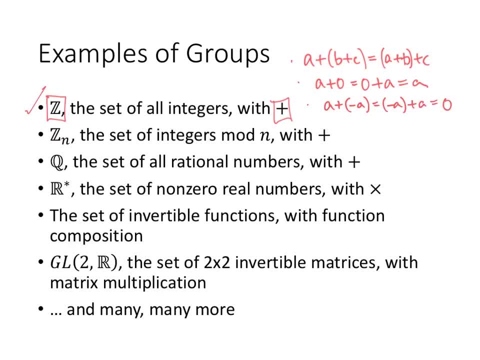 integers mod n. So again, if you're familiar with modular arithmetic, which you should be if you're watching this video, the set of all integers mod n with addition of congruence classes makes this a 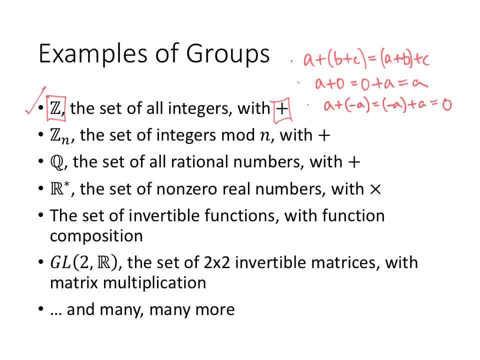 group. The set q, the set of rational numbers, that's fractions where the top and the bottom of the fraction are integers, and the bottom of course isn't zero, and I can add those rational numbers. That gives me a group as well. The set r star, the set of non-zero real numbers with 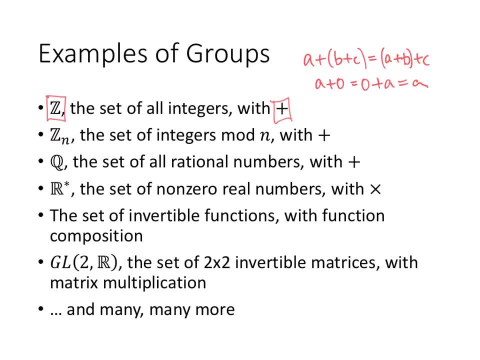 we know what that identity is. We know that identity is good ol zero. Finally, we have a requirement that we have to have an inverse for every integer And in this case, for every integer a. the inverse of a is actually negative a, because negative a plus a gives us back that identity, which is zero. 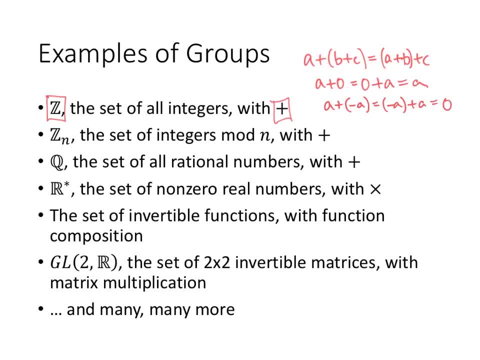 So again, I'm not calling it a to the minus 1, because in this case we specifically know that if I have any integer a, the additive inverse of that integer a is negative a. So those three lines there tell me that this is group. So I'm not going to go through and check all the properties. 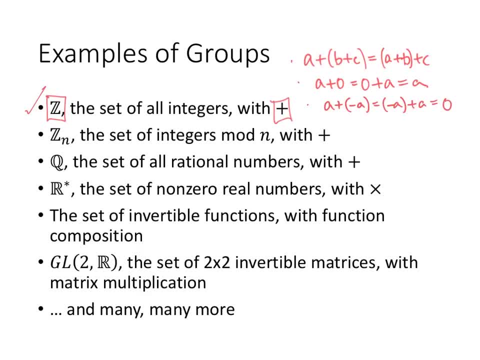 for all of these examples, but that's the idea. That's what you would have to do to verify that these things really are groups. So just going down the line here. the next example is set of integers, mod n. So, again, if you're familiar with modular arithmetic- which you should be, if you're. 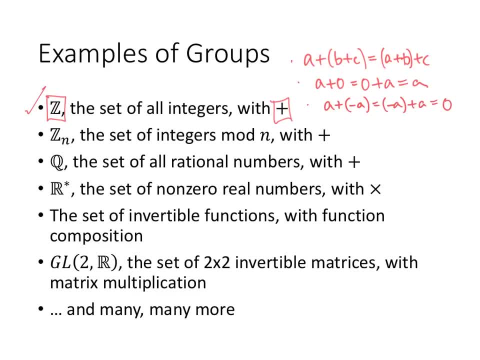 watching this video. the set of all integers, mod n, with addition of congruence classes, makes this a group. The set q, the set of rational numbers, that's fractions where the top and the bottom of the fraction are integers and the bottom of course isn't zero. and I can add those rational. 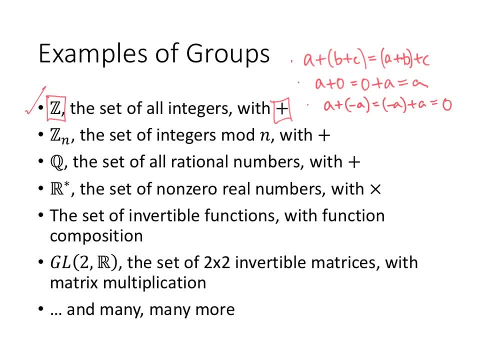 numbers. That gives me a group as well. The set r star, the set of non-zero real numbers with multiplication, is also a group. And again the identity. in this case, since the operation is multiplication, the identity would be the number one. Now notice here that this is not meant to be. 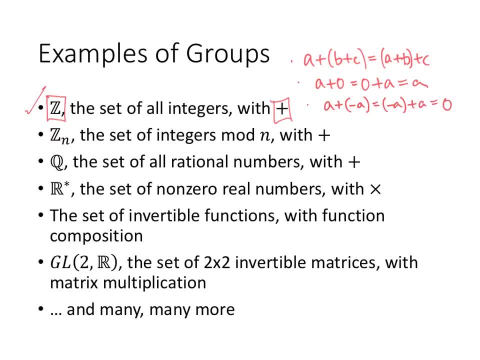 an exhaustive list. Certainly there are more things on this list. The set of non-zero rational numbers with multiplication is also a group. The set of real numbers with addition is also a group. So there's lots and lots and lots of examples. Another different kind of example is the set of 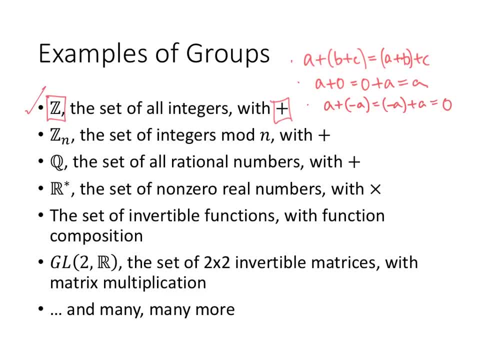 invertible functions with function composition. So if I compose functions, that operation is associative. So f composed with g composed with h is the same as f composed with g composed with h. So we've got associativity, Because I'm insisting that the functions are invertible. 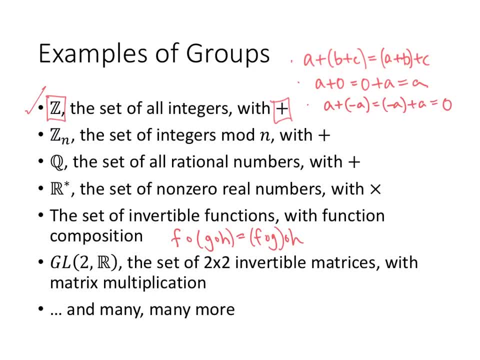 each function is going to have a number, So I'm going to have a number of numbers with an inverse, And then the identity element is actually the identity function, which we might call i, And this function just has the boring formula that i of x equals x for all x Another. 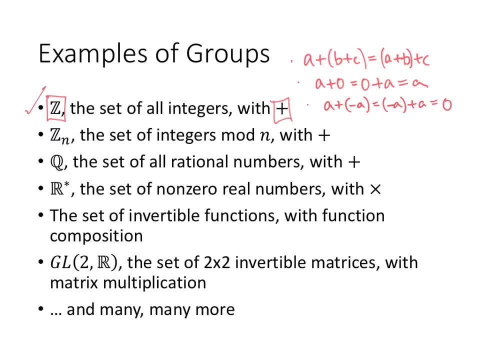 multiplication, is also a group. And again, the identity in this case, since the operation is multiplication, the identity would be the number one. Now notice here that this is not meant to be an exhaustive list. Certainly there are more things on this list. The set of non-zero rational numbers. 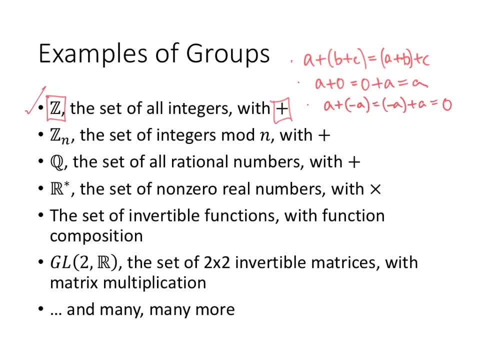 with multiplication is also a group. The set of real numbers with addition is also a group. So there's lots and lots and lots of examples. Another different kind of example is the set of 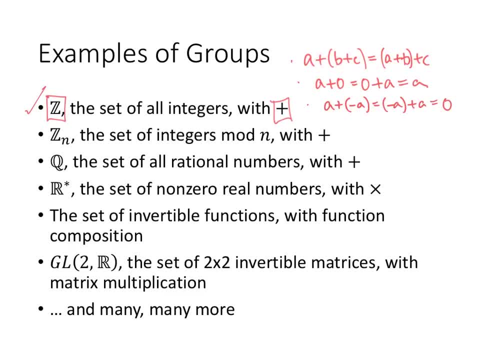 invertible functions with function composition. So if I compose functions, that operation is associative. So f composed with g composed with h is the same as f composed with g composed with h. 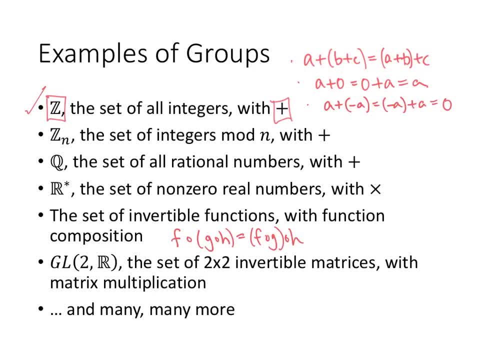 So we've got associativity. Because I'm insisting that the functions are invertible, each function is going to have a number. So I'm going to have a number of numbers with an inverse. And then the identity element is actually the identity function, which we might call i. And this function just has the boring formula that i of x equals x for all x. Another 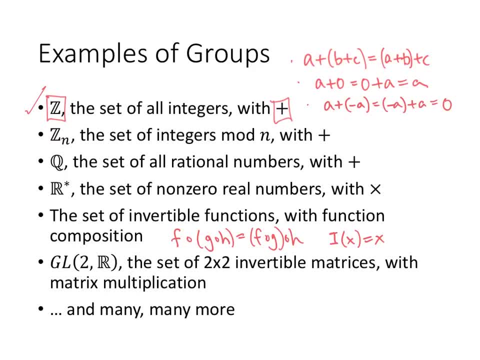 different kind of example is a set of two-by-two invertible matrices with matrix multiplication. 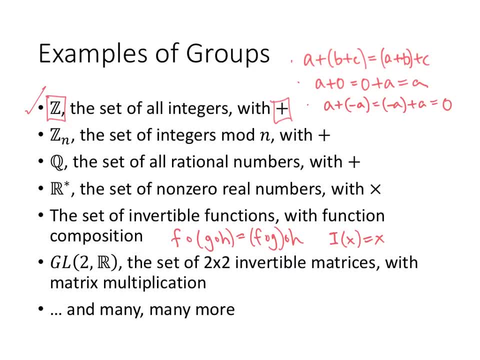 So again, I'm insisting on the matrices being invertible so that I get that inverse requirement for being a group. The identity element is going to be the identity matrix. And then we know that matrix multiplication is not necessarily always commutative. So I'm going to have a number of matrices with matrix multiplication. So f is associative. a times b is not always equal to b times a. But it is associative, because if I have three matrices, a, b, and c, a times b times c like that is the same as a times b times c like that. But a times b is not always equal to b times a. So not always, anyway. So when a group has that additional property, when a times b is not always equal to b times a, we say that it's a commutative group, or sometimes an abelian group. 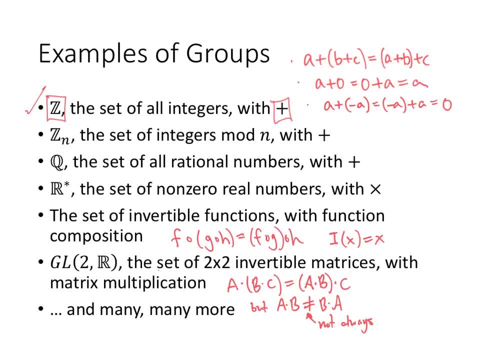 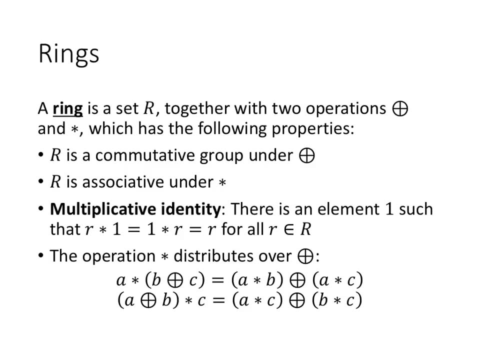 But a group does not require that commutativity. So you're still allowed to be a group even if a times b does not always equal b times a. So some of these examples are abelian groups, are commutative groups, but some of them are not. So our next example of an algebraic structure is 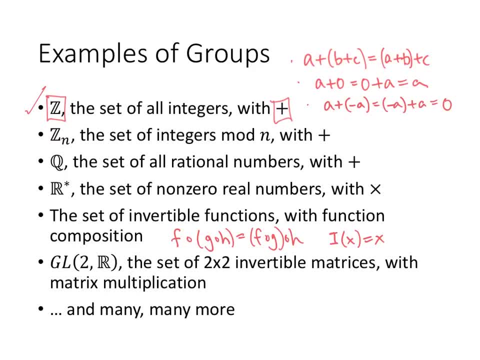 different kind of example is a set of two-by-two invertible matrices with matrix multiplication. So again I'm insisting on the matrices being invertible so that I get that inverse requirement for being a group, The identity element is going to be the identity matrix, And then we know that. 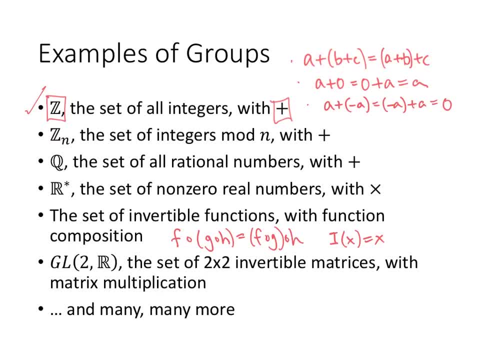 matrix. multiplication is not necessarily always commutative. So I'm going to have a number of functions with function composition. So if I have a group that is associative, a times b is not always equal to b times a, But it is associative because if I have three matrices- a, b and c- a times b. 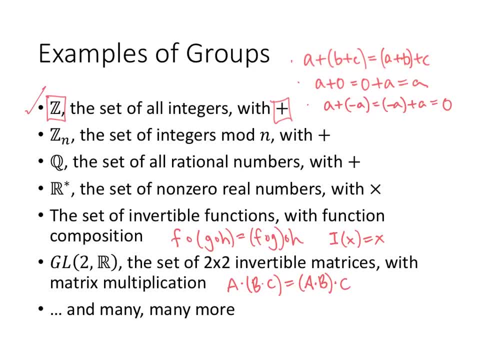 times c like that is the same as a times b times c like that. But a times b is not always equal to b times a, So not always anyway. So when a group has that additional property, when a times b is always equal to b times a, we say that it's a commutative group or sometimes an abelian group. 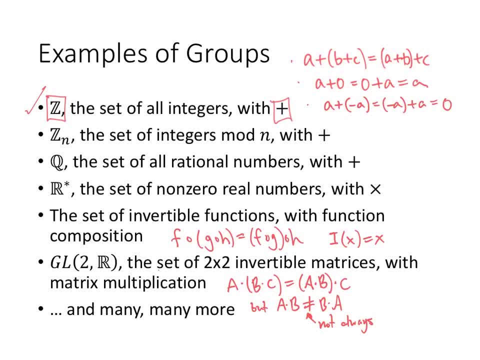 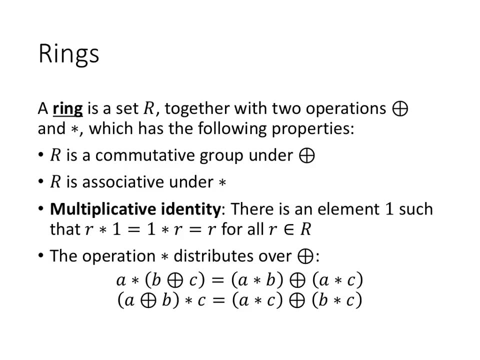 But a group does not require that commutativity, So you're still allowed to be a group, even if a times b does not always equal b times a. So some of these examples are abelian groups are commutative groups, but some of them are not. So our next example of an algebraic structure is: 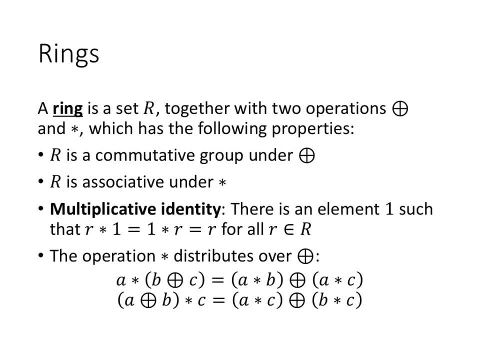 a ring. So this is a little bit more complicated than a group. In this case we have two operations, which I'm calling the same, plus in a circle thing, and then star, And so we think of those as being addition and multiplication. So again, I've chosen symbols that are reminiscent of those symbols that we're used. 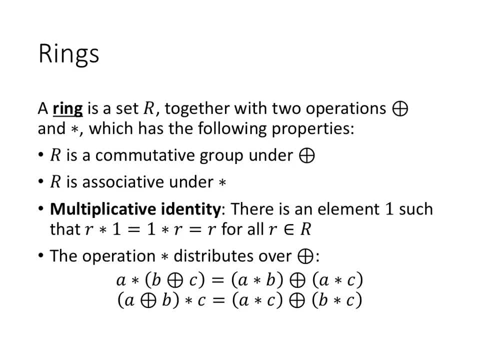 to, but not necessarily the exact symbols that we normally use. So what do we have for it to be a ring? Well, again, using some of the terminology that we've already developed, one of the requirements is that r has to be a commutative ring under that addition property. So in this, 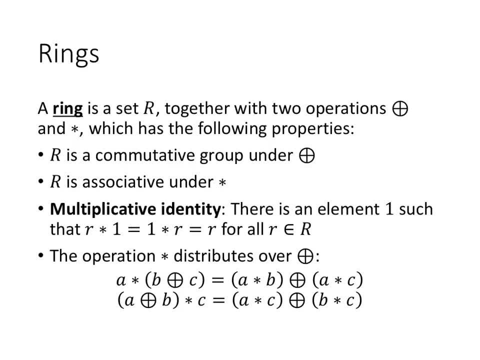 case, that means there's an additive identity, there are additive inverses and that addition is both associative and commutative. So all of those things have to be true. Now getting to the star, the star operation, multiplication has to be associative. There has 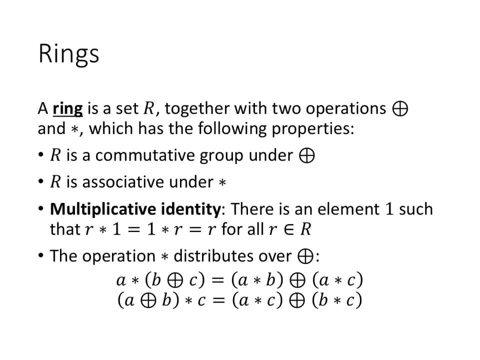 a ring. So this is a little bit more complicated than a group. In this case, we have two operations, which I'm calling, this is the same plus in a circle thing, and then star. And so we think of those as being addition and multiplication. So again, I've chosen symbols that are reminiscent of those symbols that we're 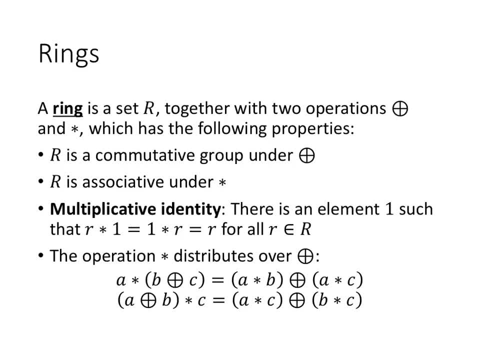 used to, but not necessarily the exact symbols that we normally use. So what do we have to be a ring? Well, again, using some of the terminology that we've already developed, one of the requirements is that r has to be a commutative ring under that addition property. So in this case, that means there's an additive identity, there are additive inverses, and there's an associative and commutative. So all of those things have to be true. Now getting to the star, the star operation, multiplication, has to be associative. There has to be a multiplicative identity. And since it's a multiplicative identity, we usually call it one, even though it might not actually be the real number one that we're used to. So that's a little bit of a notational thing. And then finally, the multiplication and addition operations interact with each other in the way that we would expect them to interact with each other. 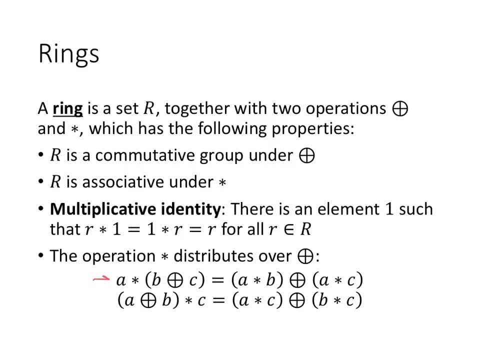 In other words, we have distributivity, which we have left distributivity here, and right distributivity there, because the star operation, the multiplication, does not have to actually be commutative. Again, a times b does not always have to equal b times a. Now something to note here, you may have seen this property here, this multiplicative identity missing. It really is standard for a ring to be required to have a multiplicative identity. 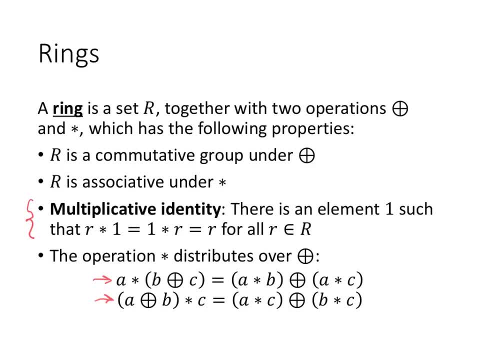 Sometimes you'll see that we might care about a situation where we have all of the rest of these properties, but we just don't happen to have a multiplicative identity. Some people give this type of structure where we have everything for a ring except a multiplicative identity. Some people will call these RNG, where we write the word ring, but we leave out the I. 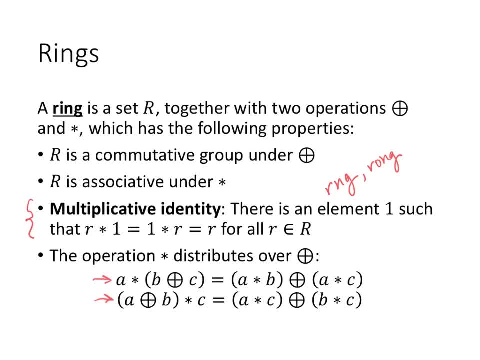 I've also seen this called a wrong, R-O-N-G, because it's wrong for a ring to not have a one element. 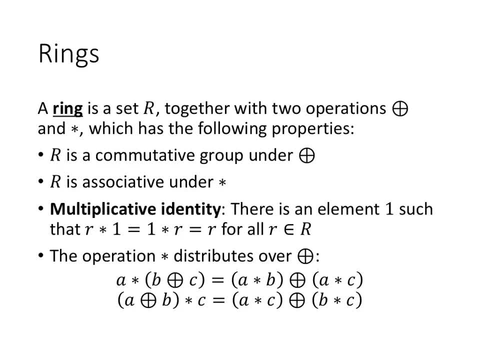 to be a multiplicative identity, and since it's a multiplicative identity, we usually call it one, even though it might not actually be the real number one that we're used to, So that's a little bit of a notational thing. And then, finally, the multiplication and addition operations interact. 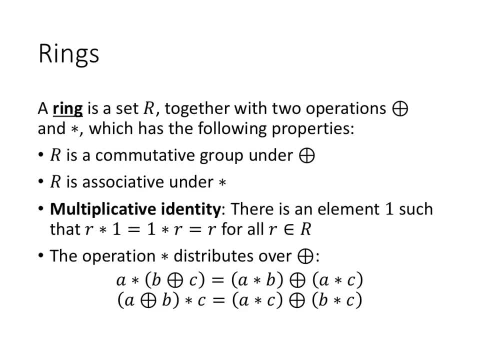 with each other in the way that we would expect them to be. So we have a multiplication and addition. In other words, we have distributivity which we have left, distributivity here and right distributivity there, because the star operation, the multiplication, does not have to actually be. 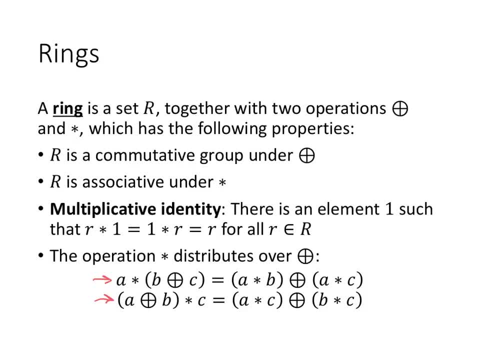 commutative. Again, a times b does not always have to equal b times a. Now something to note here. you may have seen this property here, this multiplicative identity missing. It really is standard for a ring to be required to have a multiplicative identity. 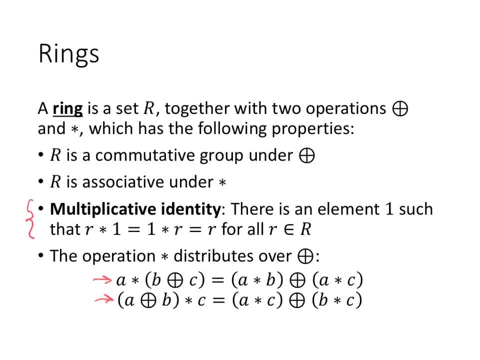 but sometimes you'll see that we might care about a situation where we have all of the rest of these properties but we just don't happen to have a multiplicative identity. Some people give this type of structure where we have everything for a ring except a multiplicative identity. 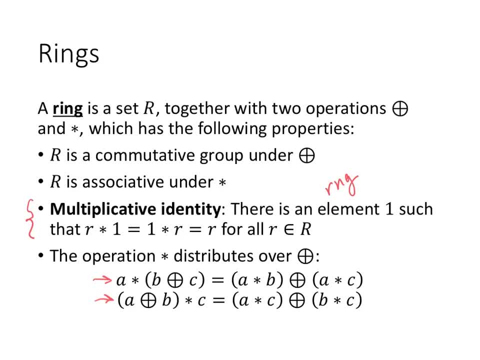 Some people call these RNG, where we write the word ring but we leave out the I. I've also seen this called a wrong R-O-N-G, because it's wrong for a ring to not have a one element. So there are reasons for that. There are reasons for that. There are reasons for that. There are. 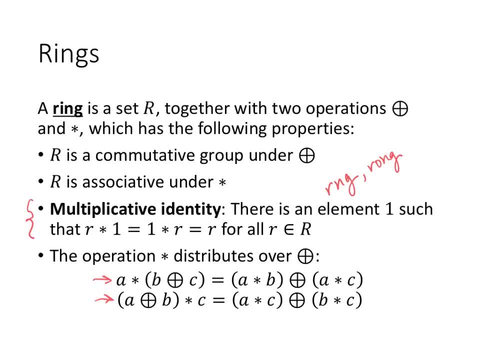 reasons why we might study something that has all of the properties of a ring without the multiplicative identity. but it really is standard to require the multiplicative identity to be there for this to be considered a ring. So if we leave this property out, then we have again a ring. 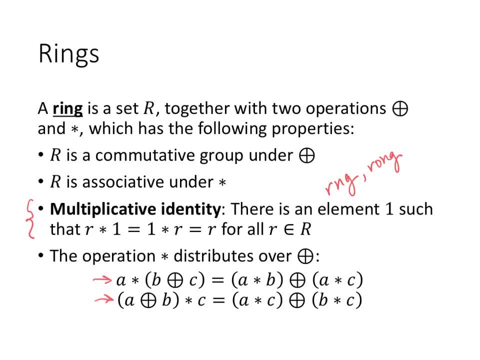 So there are reasons for this. Reasons why we might study something that has all of the properties of a ring without the multiplicative identity, but it really is standard to require the multiplicative identity to be there for this to be considered a ring. So if we leave this property out, then we have, again, a ring 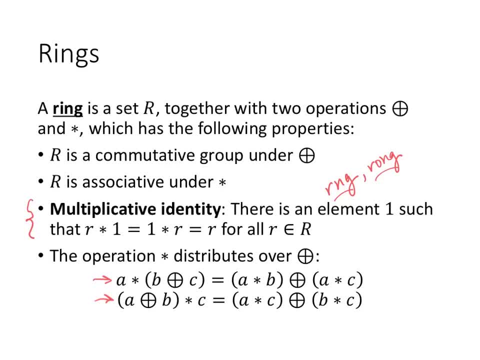 with no I, or a wrong with an O instead of an I. That's if you have everything except multiplicative 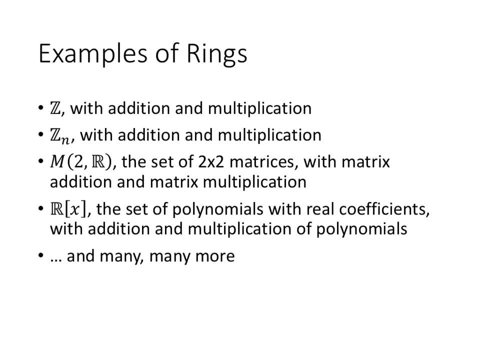 identity. So again, there's lots of examples of rings. So again, for it to be a ring, you have to have an addition and an addition. So if you have an addition and an addition, you have to have an addition and a multiplication, and those addition and multiplication have to have lots of different properties. So to actually verify that something is a ring would be quite involved. 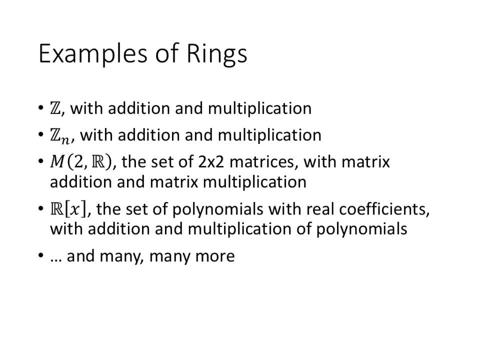 You'd have to demonstrate a lot of different properties. I'm not going to go through those 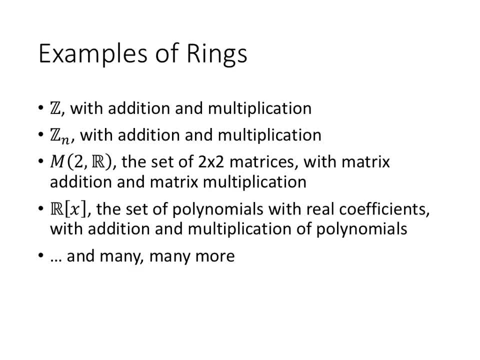 details here, but just to give you an idea, that would be a lot of work. So the set of integers 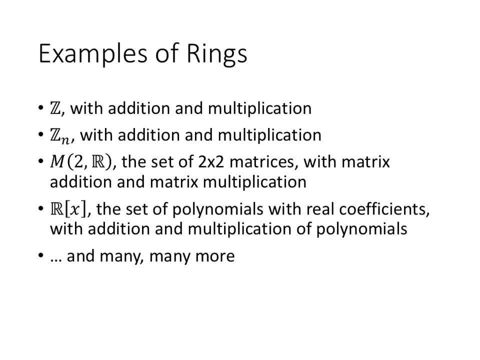 with addition and multiplication is a ring. The set of integers mod N is also a ring. The set of all two by two matrices. So the matrices don't have to be invertible, because to be invertible, you don't have to be a ring. You don't have to have multiplicative inverses. You do have to have additive inverses, but the additive inverse of a matrix is just what you get by putting minus signs in front of every entry of the matrix. So that turns out to be a ring. Another good example of a ring is a set of polynomials. So this R brackets X here, that's notation for the set of all 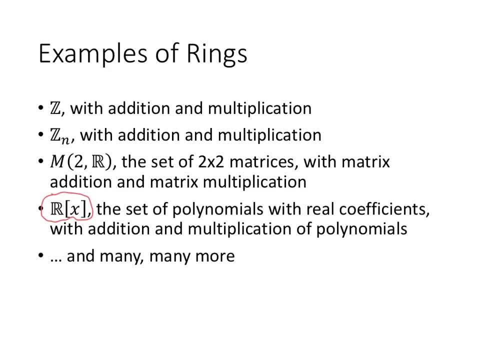 polynomials with real coefficients. And again, we can add and multiply polynomials. And as I've said before, there's lots and lots and lots and lots of examples of these. These are all polynomials, but these are just a few. Again, we're just trying to get an overview here, trying to scratch the surface of these different kinds of algebraic structures. 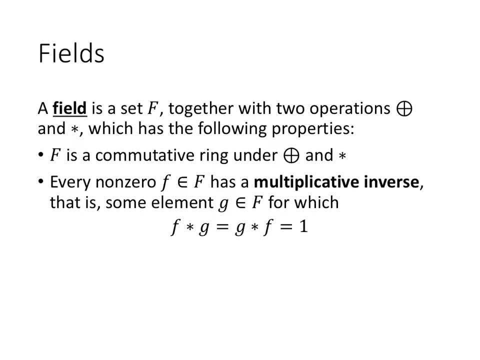 Next up in our discussion of algebraic structures, a little bit more complicated, is something called 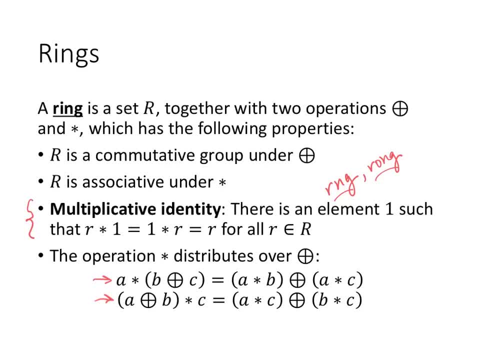 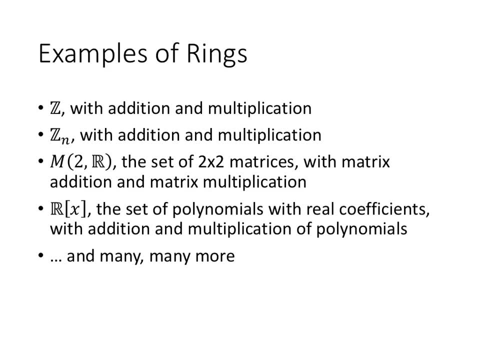 with no I or a wrong with an O instead of an I, That's if you have everything except multiplicative identity. So again, there's lots of examples of rings. So again, to be a ring you have to have a ring and a multiplication, and those addition and multiplication have to have lots of different. 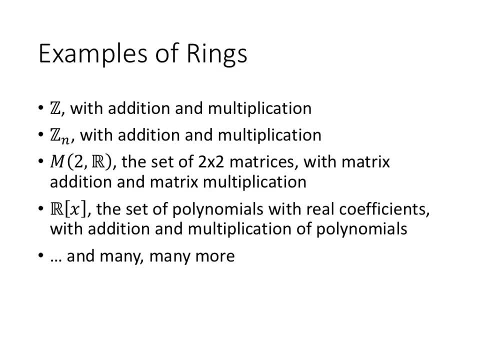 properties. So to actually verify that something is a ring would be quite involved. You'd have to demonstrate a lot of different properties. I'm not going to go through those details here, but just to give you an idea. that would be a lot of work. So the set of integers with addition and 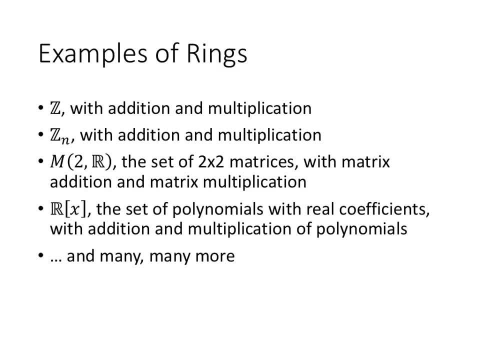 multiplication is a ring. The set of integers, mod N is also a ring, The set of all 2x2 matrices. so the matrices don't have to be invertible, because to be a ring you don't have to have multiplicative inverses, You do have to have additive inverses. 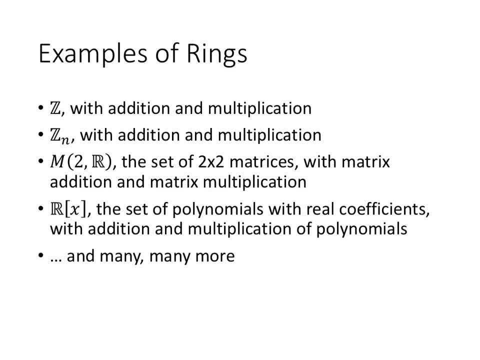 but the additive inverse of a matrix is just what you get by putting minus signs in front of every entry of the matrix, So that turns out to be a ring. Another good example of a ring is a set of polynomials. So this R brackets X here. that's notation for the set of all polynomials. 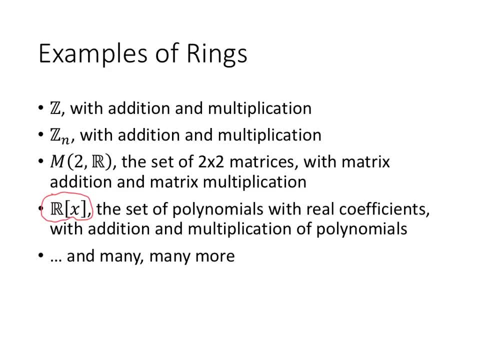 with a real coefficients. And again we can add and multiply polynomials And, as I've said before, there's lots and lots and lots and lots of examples of these. These are just a few. Again, we're just trying to get an overview here, trying to scratch the 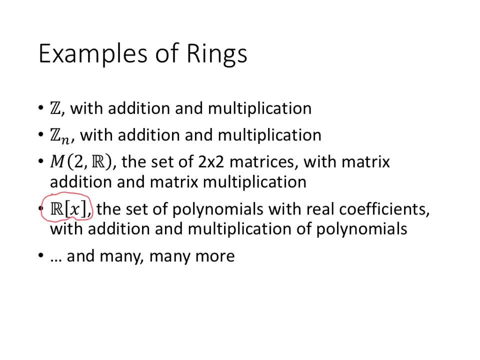 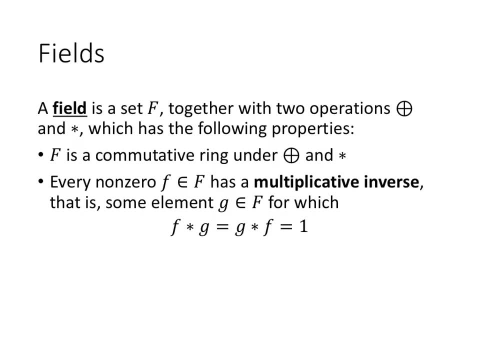 surface of these different kinds of algebraic structures. Next up in our discussion of algebraic structures, a little bit more complicated, is something called a field. So a field is very similar to a ring. We've got two operations: addition and multiplication, And now that we've 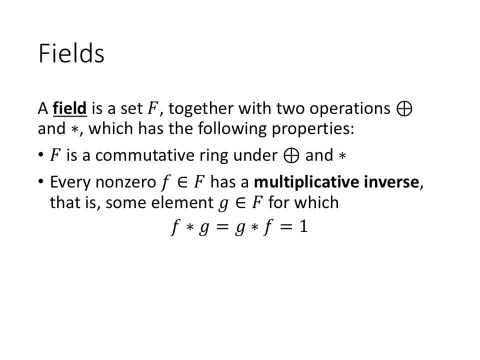 established some of this terminology. we can describe a field by saying that this field is a commutative ring under addition and multiplication. So now, when I say commutative ring, I'm talking about the multiplication being commutative. A ring. to be a ring, the multiplication does not have to be commutative, But to be a field, 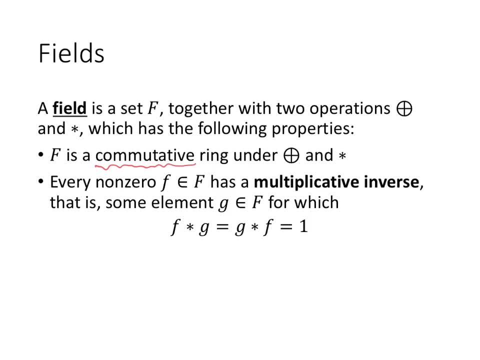 the multiplication does have to be commutative. And then, finally, the property to be a field is that we have to have multiplicative inverses for every element of this field other than zero. So for every f not zero, there's some other element, g, so that f times g is the same as g times f. 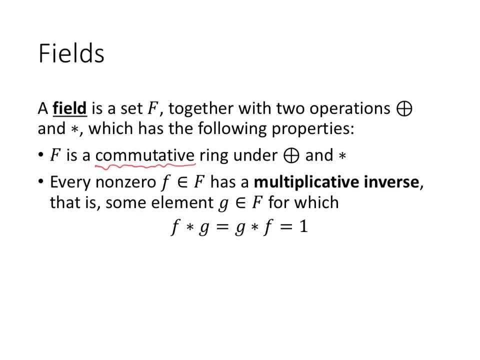 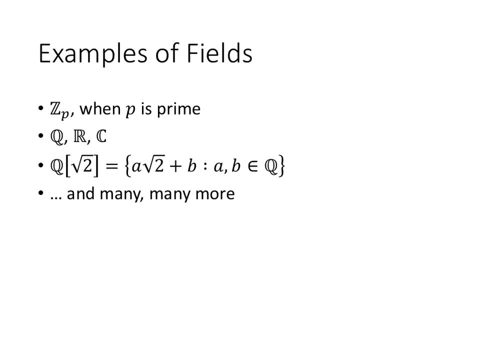 because the multiplication is commutative And that gives me one, the multiplicative identity. So a field you can think of as a ring, where the multiplication is commutative and every element has a multiplicative inverse other than zero. As usual, lots of examples of fields, some of which are familiar to us: Integers mod p. 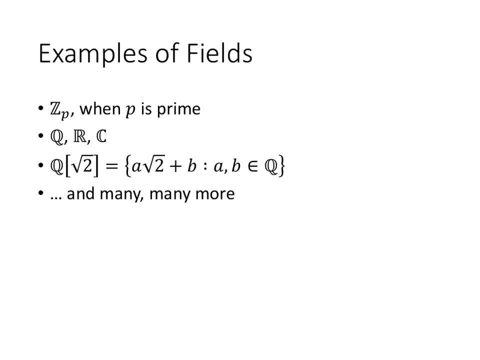 where p is prime is an example of a field. If you're looking at integers mod n and n is not prime, then not every element of that ring will have a multiplicative inverse. But when p is prime, it's a multiplicative inverse. So if you're looking at an element of this ring, you'll have a multiplicative. 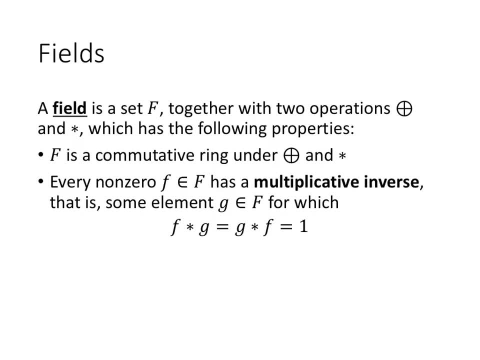 a field. So a field is very similar to a ring. We've got two operations, addition and multiplication. So, and now that we've established some of this terminology, we can describe a field by saying that this field is a commutative ring under addition and multiplication. So now when I say commutative ring, I'm talking about the multiplication being commutative. A ring, to be a ring, the multiplication does not have to be commutative. But to be a field, the multiplication does have to be commutative. And then finally, the property to be a field is that we have to have multiplicative inverses for every element of this field other than zero. So for every f not zero, there's some other element g, so that f times g is the same as g times f, because the multiplication is commutative. 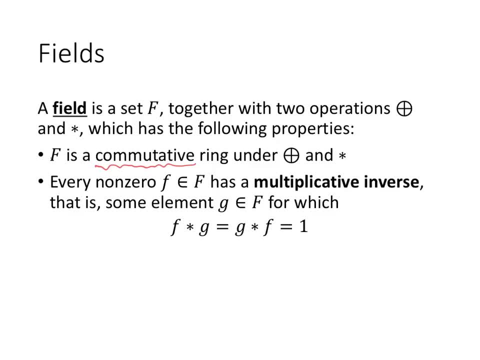 And that gives me one, the multiplicative identity. So a field you can think of as a ring, where the multiplication is commutative, and every element has a multiplicative inverse other than zero. 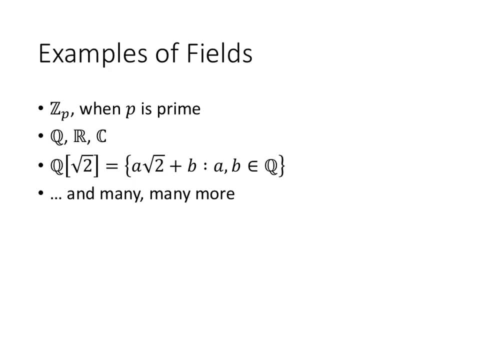 As usual, lots of examples of fields, some of which are familiar to us. Integers mod p, where p is prime, is an example of a field. If you're looking at integers mod n, and n is not prime, then not every element of that ring will have a multiplicative inverse. But when p is prime, then everything other than zero will have a multiplicative inverse. 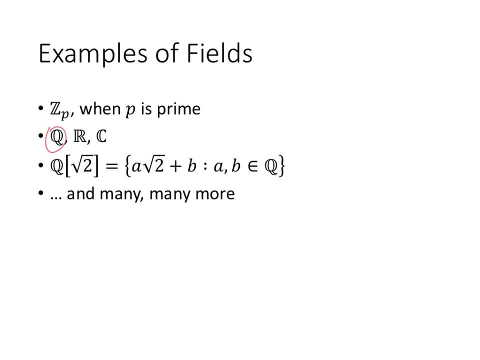 Again, other common examples are q, the set of rational numbers. Remember, that's fractions, where the top and the bottom are whole numbers. r, the set of real numbers. c, we haven't seen this yet in this video, but c is the set of complex numbers. That's things that look like a plus bi, where i is the square root of minus one. So I'm going to spend a little bit of time talking about this last example here, which is q brackets the square root of minus one. So I'm going to spend 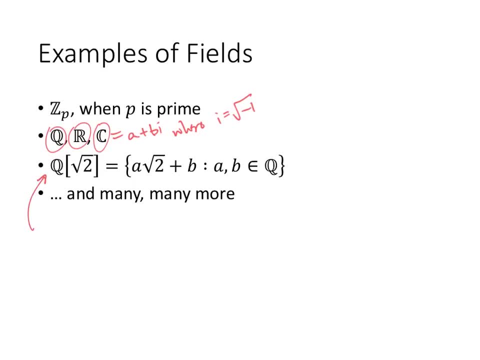 a little bit of time talking about this last example here, which is q brackets the square root of two. So this is everything that looks like a times the square root of two plus b, where a and b are rational numbers. So I just want to sort of demonstrate how these operations would work. The 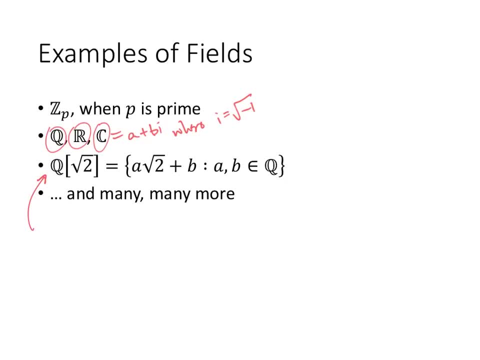 operations here are just addition and multiplication of numbers. So if I had two of these guys that I wanted to, let's say, add together, so three times the square root of two plus four, and let's say I wanted to add that to four times the square root of two plus six, I would just collect like terms. 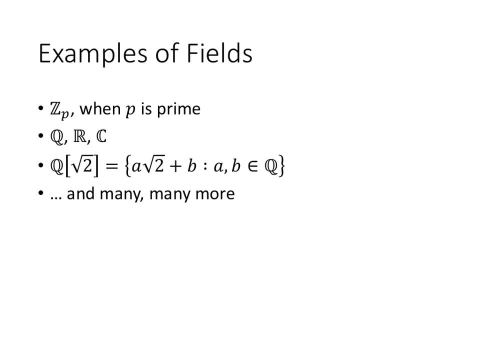 then everything other than 0 will have a multiplicative inverse Again. other common examples are: Q- the set of rational numbers, remember, that's fractions where the top and the bottom are whole numbers. R- the set of real numbers. C- we haven't seen this yet in this video, but C is the set of complex numbers. 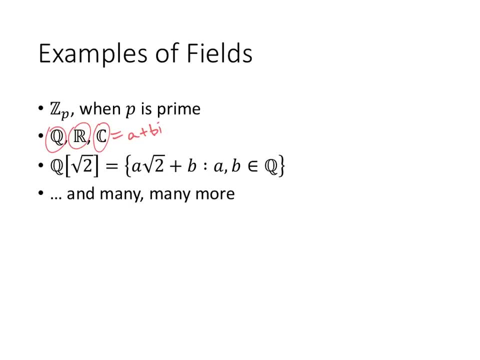 that's things that look like a plus bi, where i is the square root of minus 1.. So I'm going to spend a little bit of time talking about this last example here, which is Q brackets the square root of 2.. So this is everything that looks like a times the square root of 2 plus b, where a and b are rational numbers. 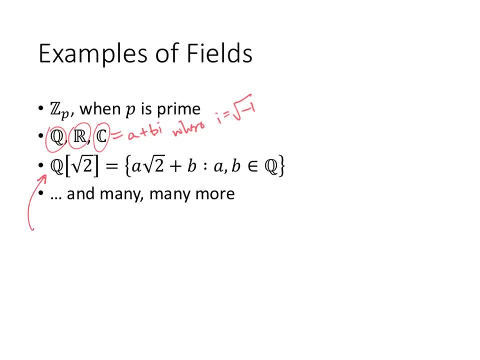 So I just want to sort of demonstrate how these operations would work. The operations here are just addition and multiplication of numbers. So if I had two of these guys that I wanted to, let's say, add together so 3 times the square root of 2 plus 4, and let's say I wanted to add that to. 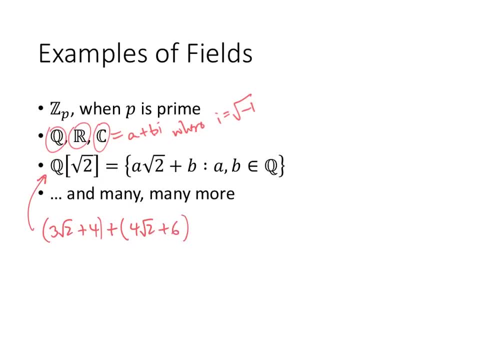 4 times the square root of 2 plus 6, I would just collect like terms, So 3 radicals, 2 plus 4 radical 2 would be 7 radical 2, and then 4 plus 6 is just 10.. 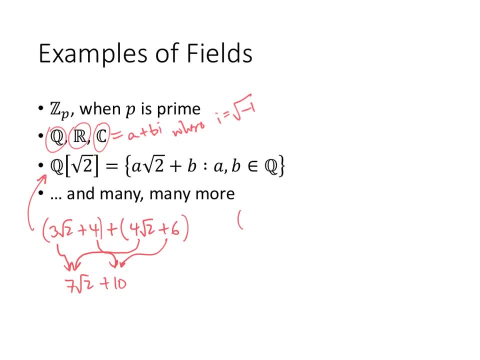 So you just add them like that. If I wanted to multiply, if I let's say I had 2 radical 2 minus 4, and then negative 5 radical 2 plus 3, and I wanted to multiply those together, 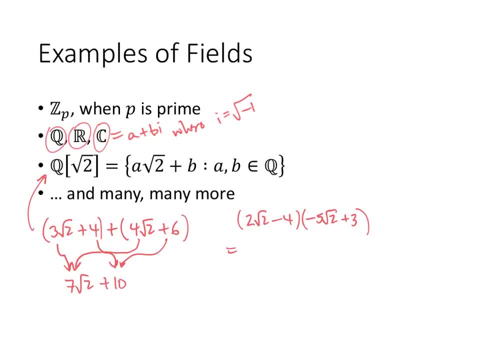 I would just use FOIL and multiply this out like I normally would. So 2 radical 2 times negative 5 radical 2 is my first. so if I'm thinking FOIL first, outer inner last, so there's my first. 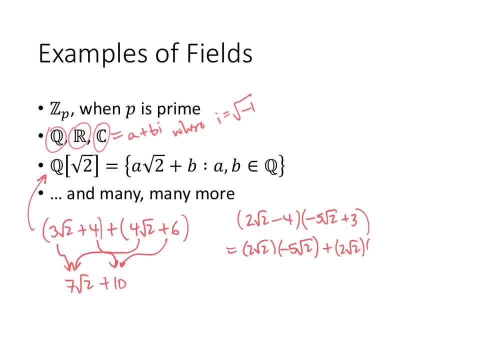 My outer is 2 radical 2 times 3.. My inner is negative 4 times negative, 5 radical 2, and my last is just negative 4 times 3.. Now I'm going to simplify these: 2 radical 2. 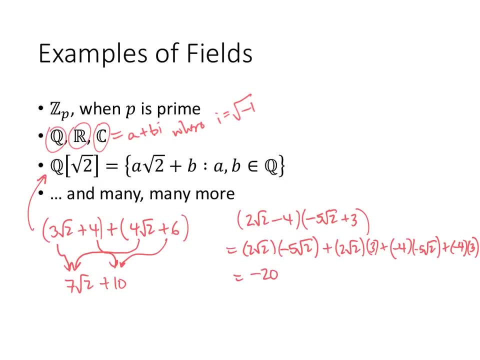 times negative: 5 radical 2 is going to be negative 20.. 2 radical 2 times 3 is going to be 6 radical 2.. Negative 4 times negative: 5 radical 2 is plus 20 radical 2, and then negative 4 times 3 is negative 12.. 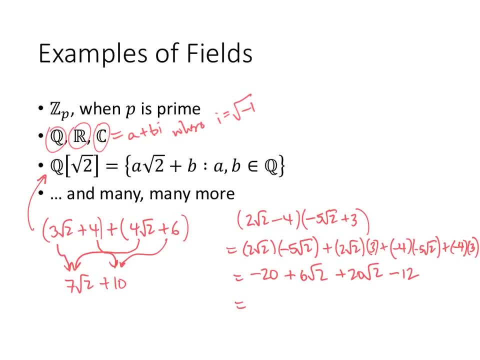 And then again I just collect like terms: So 6 radical 2 plus 20 radical 2,, that's 26 radical 2, and then negative, 20 minus 12 is minus 32.. So that's how this, this field, works, right. So that's how you add, that's how you multiply. Now it 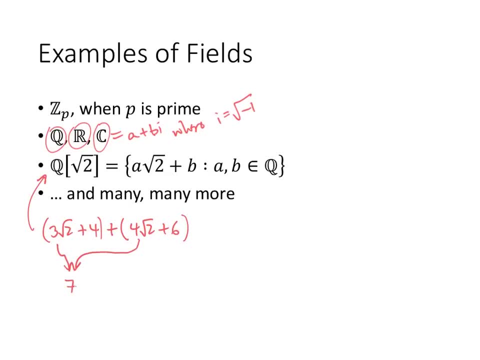 So three radical two plus four radical two, would be seven radical two, and then four plus six is just ten. So you just add them like that. 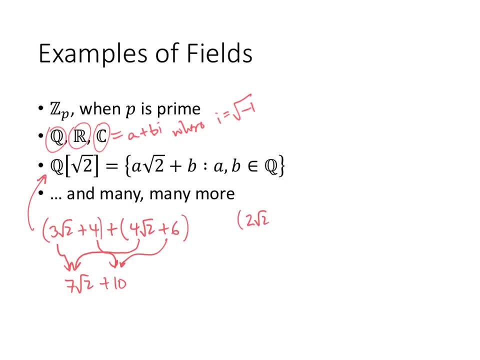 If I wanted to multiply, if let's say I had two radical two minus four, and then negative five radical two plus three, and I wanted to multiply those together, I would just use FOIL and multiply this out like I normally would. So two radical two times negative five radical two is my first, 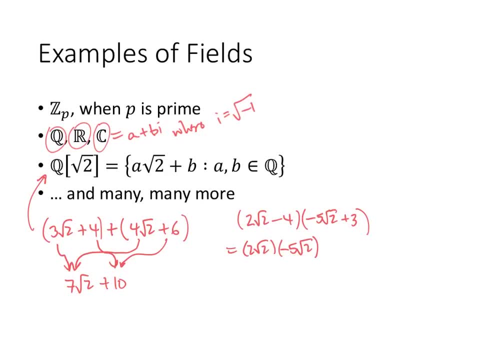 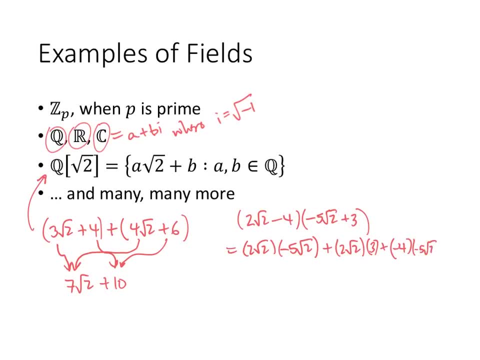 My inner is negative four times negative five radical two, and my last is just negative four times three. Now I'm going to simplify these. Two radical two times negative five radical two is going to be negative twenty. Two radical two times three is going to be six radical two. 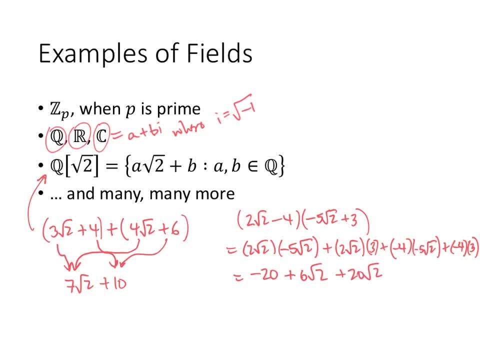 Negative four times negative five radical two is plus twenty radical two, and then negative four times three is negative twelve. And then again, 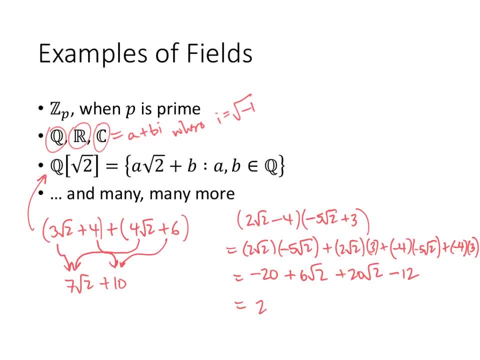 I just collect like terms. So six radical two plus twenty radical two, that's twenty-six radical two, and then negative twenty minus twelve is minus thirty-two. So that's how this field works, 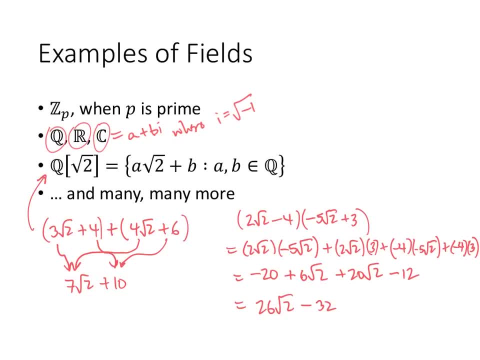 right? So that's how you add, that's how you multiply. Now it takes a little bit of thought, though, to think why is this a field? So you can maybe see all of the properties pretty clearly, 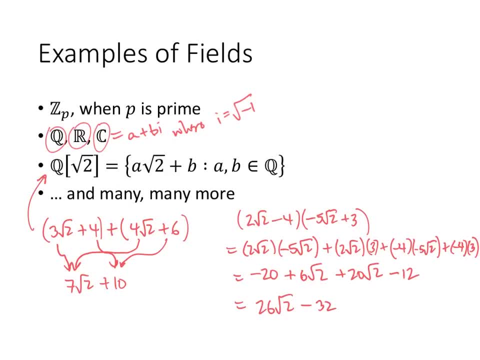 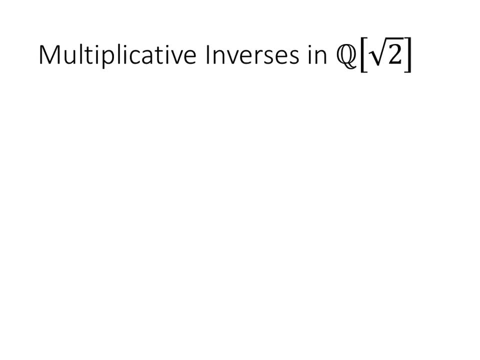 except why do we have multiplicative inverse? Why do we have multiplicative inverse? Why do we have multiplicative inverses? Why would there have to be an example that shows us why this has a multiplicative inverse? And the way that we see why there are multiplicative inverses in q brackets 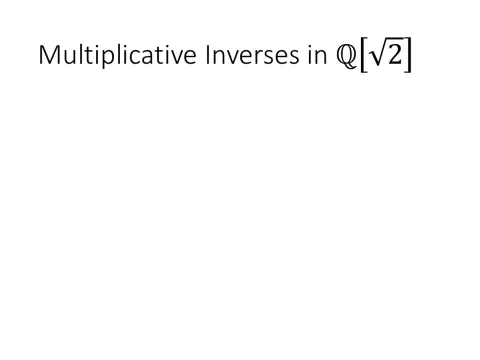 the square root of two is actually kind of clever. So what we're looking for is if I had, let's say, three radical two plus four, and I'm going to say, okay, what do I multiply that by? Some other a radical two plus b, and what I want to get back is one, right? What I want to get back 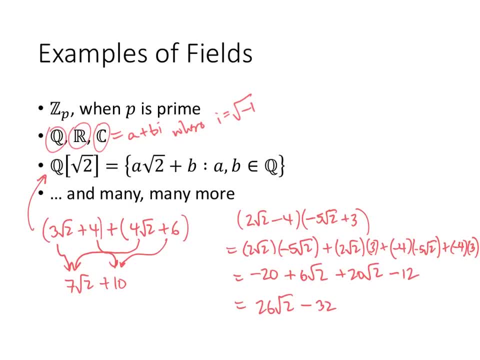 takes a little bit of thought, though, to think: why is this a field? So you can maybe see all of the properties pretty clearly, except why do we have multiplicative inverses? Why would there have to be an example that shows us why this has a multiplicative inverse? 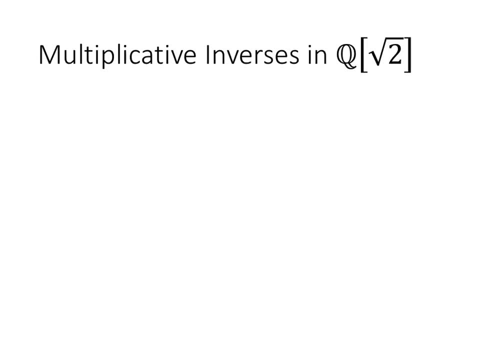 And the way that we see why there are multiplicative inverses in q brackets- the square root of 2- is actually kind of clever. So what we're looking for is if I had, let's say, 3 radical 2 plus 4, and I were to say: 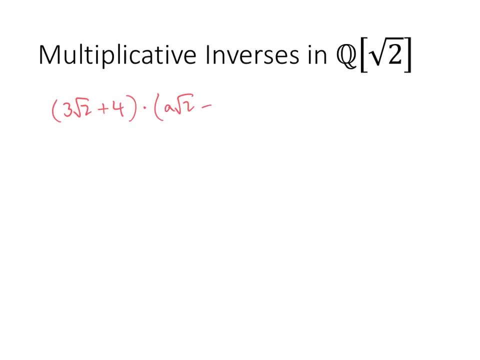 okay, what do I multiply that by Some other? a radical 2 plus b, and what I want to get back is 1, right, what I want to get back is the multiplicative identity. So what we really want to go here, 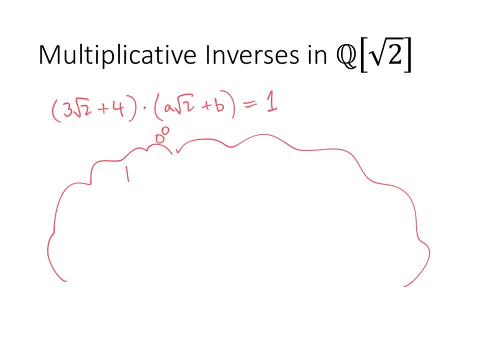 and so this is my sort of thought process. what I really want to go here is 1 over 3 radical 2 plus 4.. The only problem is that 1 over 3 radical 2 plus 4 is not of the form. 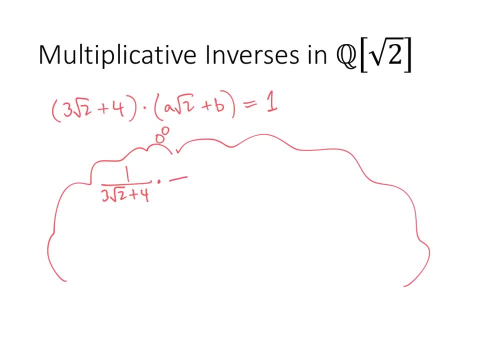 a radical 2 plus b. But I can do something kind of clever to get it into that form. What I'm going to do is multiply that fraction top and bottom by 3 radical 2 minus 4.. This is sometimes called rationalizing the denominator, something you might have done back in high. 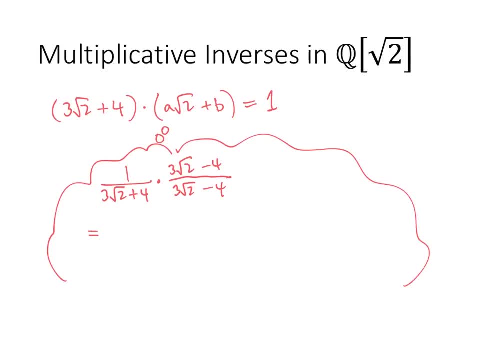 school. But when we do this, what we get is, on the top, we get 3 radical 2 minus 4.. And on the bottom, because that's a difference of two squares, we get 3 radical 2 squared minus 4 squared, And that's going to be an integer. So we get 3 radical 2 minus 4.. On 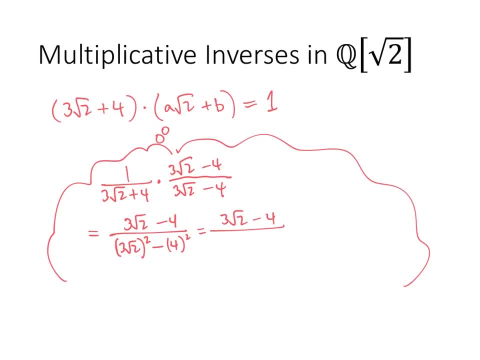 the bottom, 3 radical 2 squared is just 18.. And 4 squared is 16.. So that's just 3 radical 2 minus 4 divided by 2.. And I can write this in the form a radical 2 plus b. They're writing that as 3 halves radical 2 minus 2.. And remember: 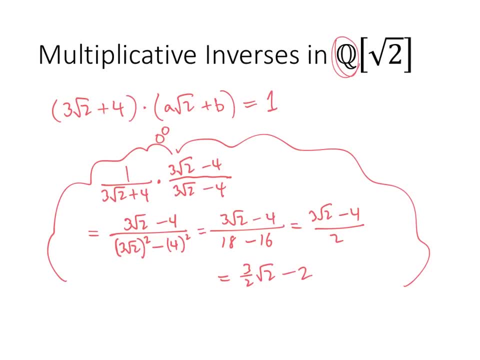 3 halves is allowed because I'm in q, I'm in rational numbers, So that's okay, And there wasn't anything special about the numbers 3 and 4 here. I could have done this with any element of q brackets to the square root of 2.. So that's really the explanation I'm 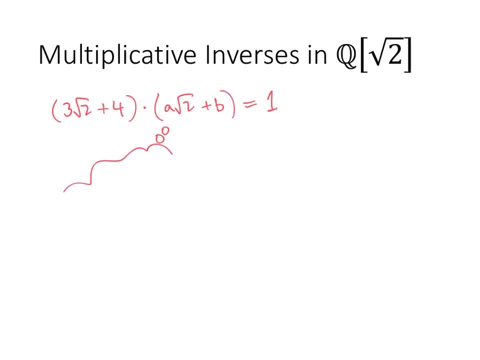 is the multiplicative identity. So what we really want to go here, and so this is my sort of thought process, what I really want to go here is one over three radical two plus four. The only problem is that one over three radical two plus four is not of the form a radical two plus b, but I can do something kind of clever to get it into that form. What I'm going to do is multiply that fraction top and bottom by three radical two minus four. This is sometimes called rationalizing the denominator, which I learned back in high school. But when we do this, what we get is on the top we get three radical two minus four, and on the bottom, because that's a difference of two squares, we get three radical two squared minus four squared, and that's going to be an integer. So we get three radical two minus four. On the bottom, three radical two squared is just 18, and that's just three radical two minus four divided by two, and I can write this in the form a radical two plus b by writing that as three halves radical two minus two. And remember, three halves is allowed, because I'm in Q, I'm in rational numbers, so that's okay. 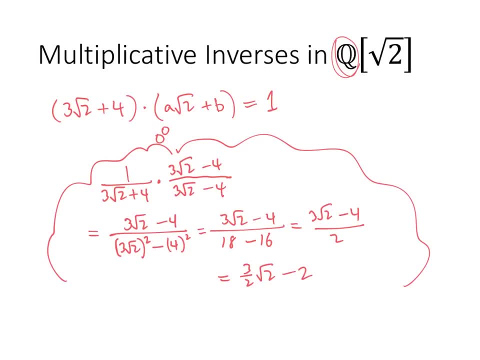 And there wasn't anything special about the numbers three and four here. I could have done this with any element of Q brackets to the square root of two. So that's really the explanation for why Q brackets the square root of two... is a field. Because everything else is pretty clear, I think, except for maybe the multiplicative inverses. But this isn't a proof, what I've written here, but this gives you the idea of 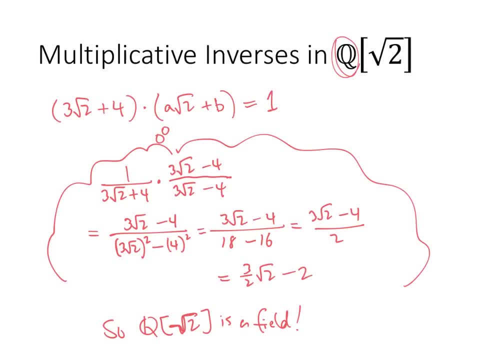 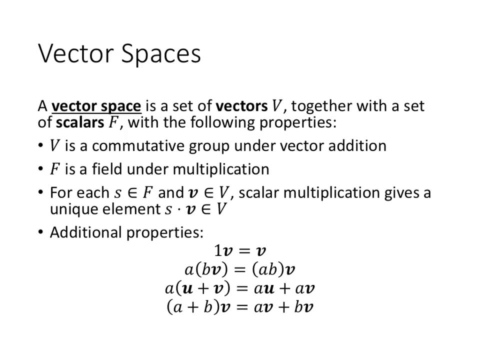 what the proof might look like of how it would justify why everything has a multiplicative inverse. Okay, I want to talk about one more type of algebraic structure that you might be 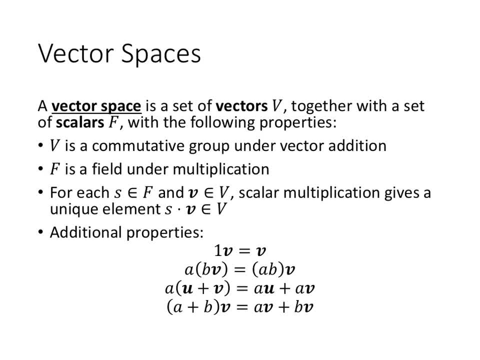 needing to know about, and that's vector spaces. So vector spaces are by far the most complicated in terms of the structure of how many things are going on, because not only do we really have two sets, we've got a set of vectors, v, and then we've also got a set of scalars, which we call f. 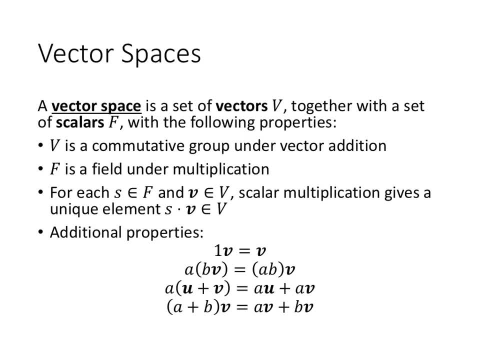 And we call it f because f is going to be required to be a field. So v is a commutative group under addition. So we've got one of our operations is vector addition. We take two things in v and add them together, and that's going to be a commutative group. 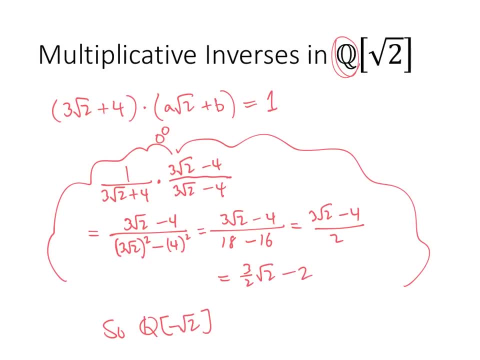 going to write the explanation for why q brackets to the square root of 2. here is a field, Because everything else is pretty clear, I think, except for maybe the multiplicative inverses. But this isn't a proof what I've written here, But this gives you the idea of what. 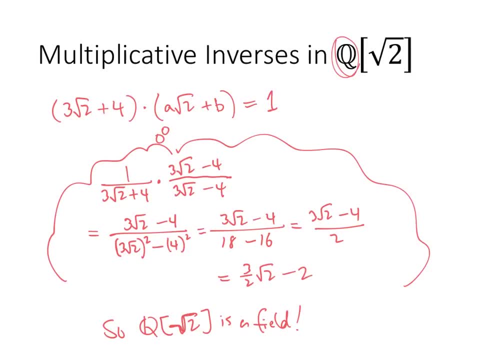 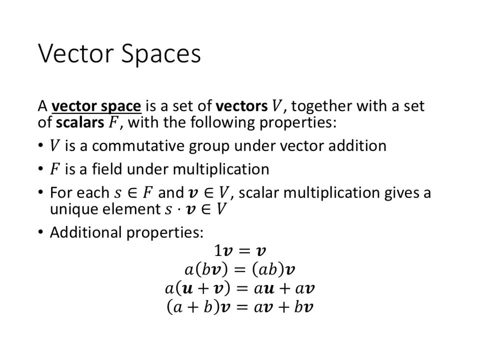 the proof might look like of how I would justify why everything has a multiplicative inverse. Okay, I want to talk about one more type of algebraic structure that you might be needing to know about Vector spaces. So vector spaces are by far the most complicated in terms of the structure. 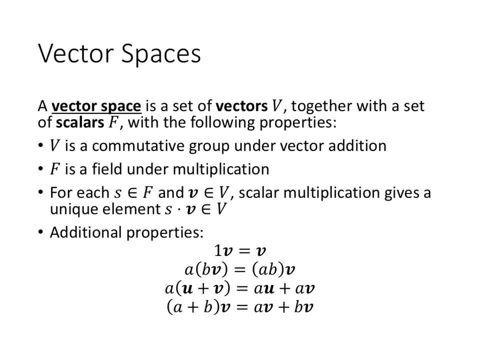 of how many things are going on, Because not only do we really have two sets, we've got a set of vectors, v, And then we've also got a set of scalars which we call f. And we call it f because f is going to be required to be a field, So v is a commutative group. 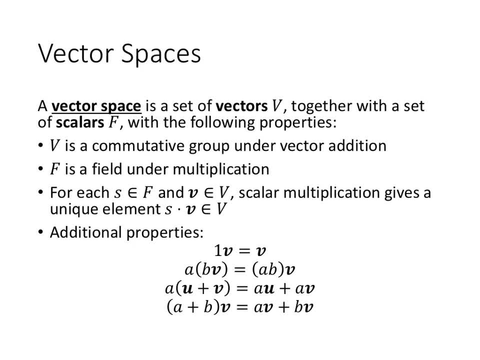 under addition. So we've got one of one of our operations is vector addition. we take two things in v and add them together And that's going to be a commutative group. So we've got- we're going to have- an identity element, the zero vector. we have inverses, additive inverses, and we have associativity. 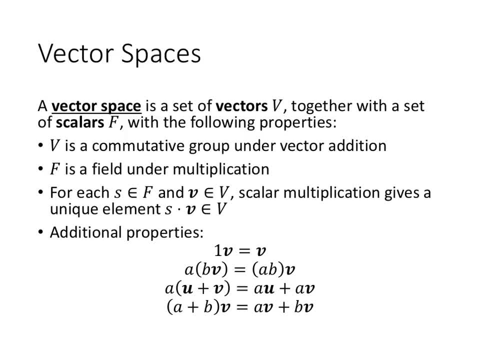 of addition and also commutativity. f by itself is a field under multiplication. So that's taking two scalars and multiplying them by each other. So we're going to have an identity scalar which is going to be the number one, or we're going to think of it as the number. 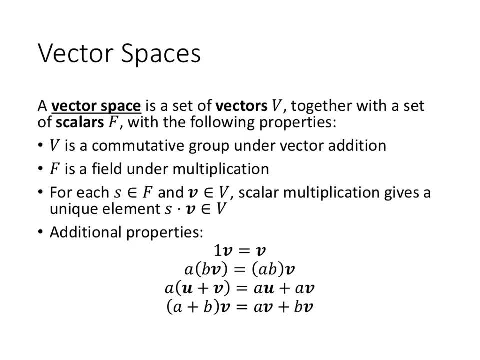 one if the field isn't numbers themselves. And then we've got an operation that lets us combine scalars and vectors, And this is a scalar multiplication. So if I've got some scalar s and some vector v, I'm going to always have to be able to. 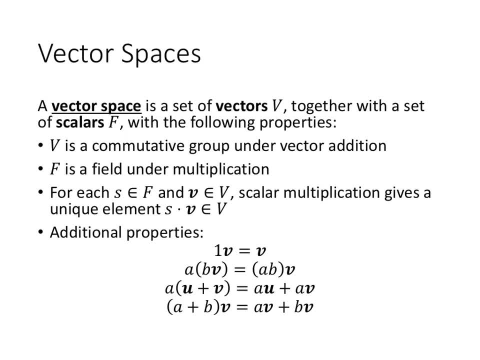 multiply that scalar by that vector And then we've got some additional properties that talk about how these things interact. So if I take the scalar one and multiply it by v, I just get v back. If I take two scalars, a times b times v should always be equal to. 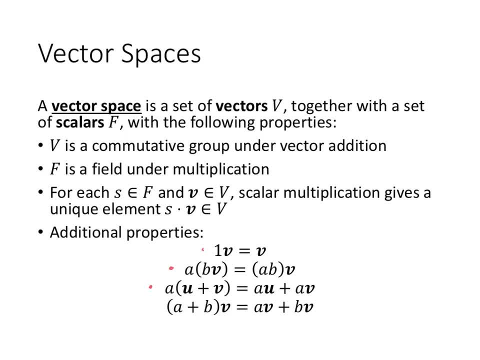 a times b, times v, And then we've got distributivity of scalar multiplication over vector addition, also of scalar multiplication across scalar addition. So it's a whole bunch of properties that when we put them all together we get this thing called a vector space. 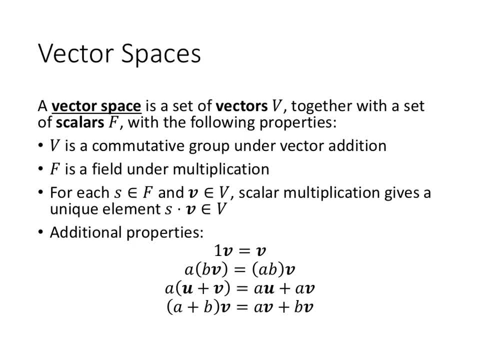 So we're going to have an identity element, the zero vector. We have inverses, additive inverses, and we have associativity of addition and also commutativity. f by itself is a field under 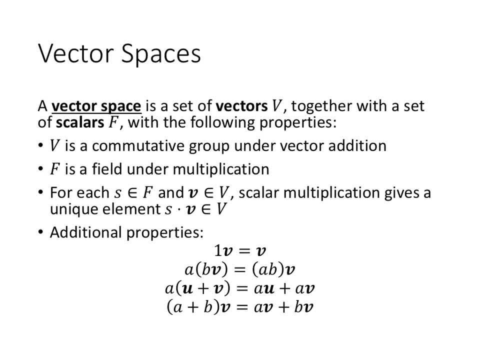 multiplication. So that's taking two scalars and multiplying them by each other. So we're going to have an identity scalar, which is going to be the number one, or we're going to think of it as the number one if the field isn't numbers themselves. And then we've got an operation that lets us combine scalars and vectors. So we're going to have an identity scalar, which is going to be 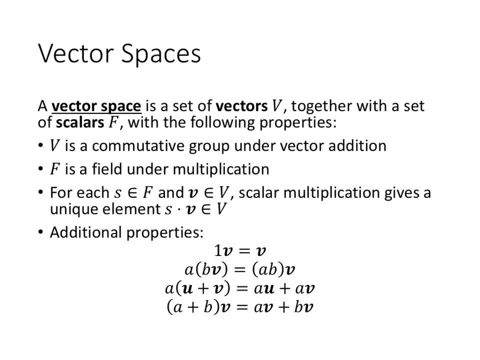 vectors. And this is a scalar multiplication. So if I've got some scalar s and some vector v, I'm going to always have to be able to multiply that scalar by that vector. And then we've got some additional properties that talk about how these things interact. So if I take the scalar one and multiply it by v, I just get v back. If I take two scalars, a times b times v should always be equal to a times b times v. And then we've got distributivity of scalar multiplication over vector 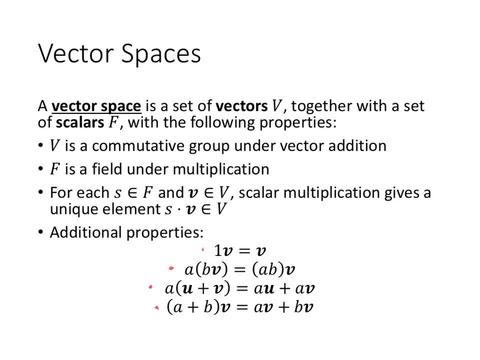 and also of scalar multiplication across scalar addition. So it's a whole bunch of properties 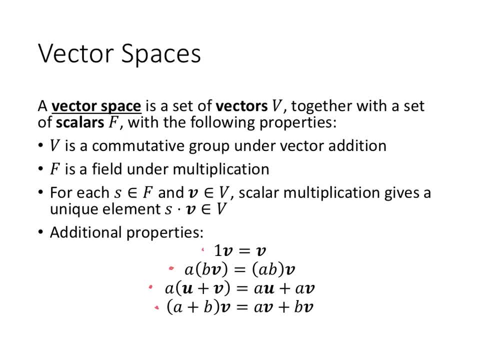 that when we put them all together, we get this thing called a vector space. 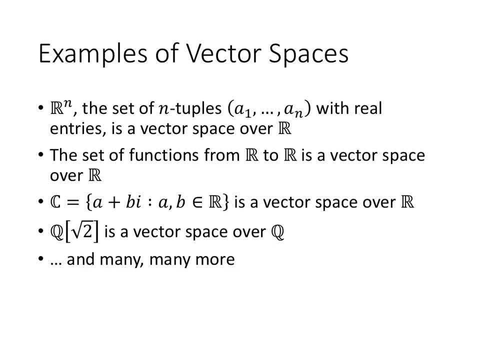 So we've got lots of examples of vector spaces. Probably if you've ever seen vector spaces before, the one that you're most familiar with is this thing rn, which is the set of n tuples. Sometimes we can think of these as column vectors. You might be more familiar with them in this form. So a1 through an. So a list of numbers, in this case real numbers, and that's going to be a vector space over the set of reals. I can add two vectors, and that's a commutative group under that operation. The scalars themselves, r is a field under the normal real number operations. And then we can also multiply any vector by a scalar. Another example that might be a little bit less familiar is the set of functions from the real numbers to the real numbers. Think calculus functions here. So a function that when I plug in a real number, I get back a real number. And that's going to be a vector space over the set of reals. And that's going to be a vector space over the set of reals. And that's going to be a set of real numbers. Again, just briefly, I can add two functions. I can multiply a function by a scalar and get another function. So that gives me a vector space. The set of complex numbers is also can be thought of as a real vector space. Now, I'm skipping some of the operations, 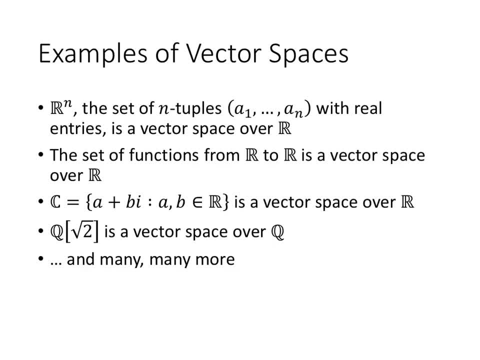 So we've got lots of examples of vector spaces. Probably, if you've ever seen vector spaces before, the one that you're most familiar with is this thing: Rn, which is the set of n tuples. Sometimes we can think of these as column vectors. You might be more familiar with them in this form. 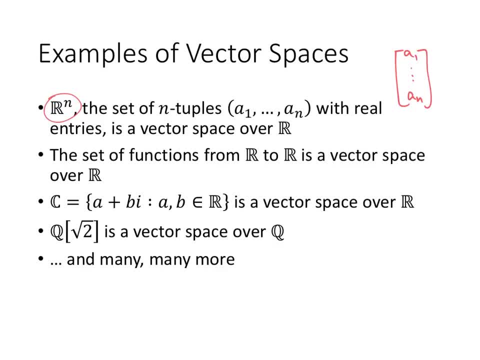 So a1 through an. So it's just a list of numbers, in this case real numbers, and that's going to be a vector space over the set of reals. I can add two vectors and that's a commutative group. under that operation, The scalars themselves, R is a field. 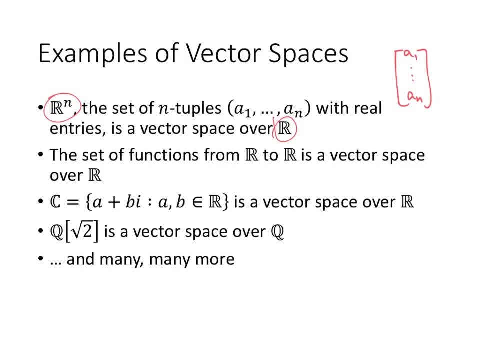 under the normal real number operations, and then we can also multiply any vector by a scalar. Another example that might be a little bit less familiar is the set of functions from the real numbers to the real numbers. Think calculus functions here. So a function that when I plug 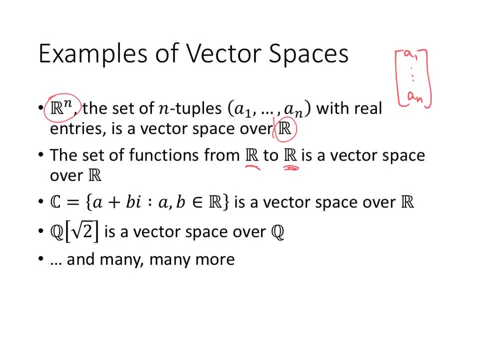 in a real number, I get back to the real number So I can add a function to the real number and that's going to be a vector space over the set of real numbers. Again, just briefly, I can add two functions. I can multiply a function by a scalar and get another function, So that gives. 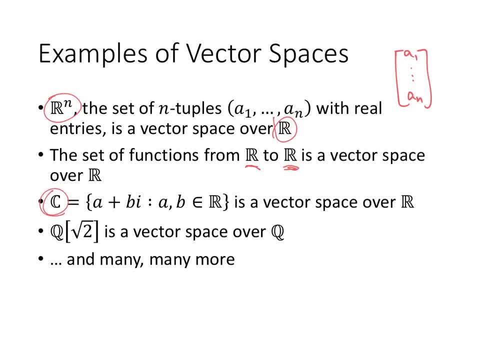 me a vector space, The set of complex numbers also can be thought of as a real vector space. Now I'm skipping some of the operations, right. So this set C, if I think of it as a vector space, I'm ignoring some of the operations that can be done on complex numbers. So when we think of a 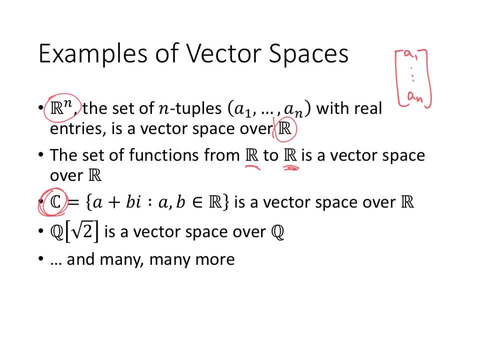 vector space. we think of it as a vector space, So I'm ignoring some of the operations that can be done on complex numbers. We think of adding two vectors together. We think of multiplying a vector by a scalar, But if my vectors are complex numbers, it's actually possible to multiply two. 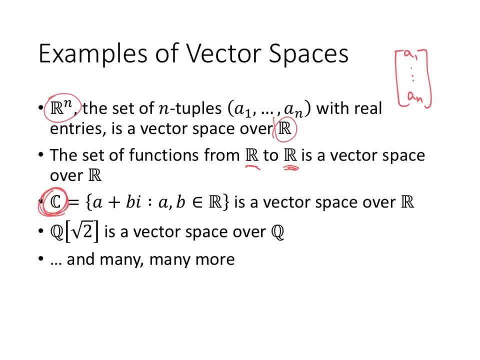 complex numbers and that operation also has a bunch of cool properties. But if I'm thinking of it as a vector space, I'm ignoring that operation that I can do of multiplying two vectors together. So in a vector space, if you have the ability to multiply two vectors together, you just ignore. 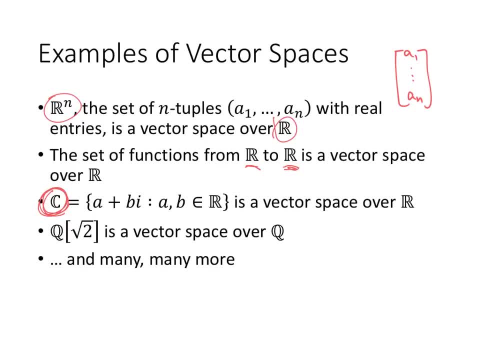 that You pay no attention to that. Another example that's going to be a little bit more kind of like the complex numbers is this thing: q squared of 2 that we were talking about. Again, I have the ability to multiply two of those vectors together, but when we think of it as a 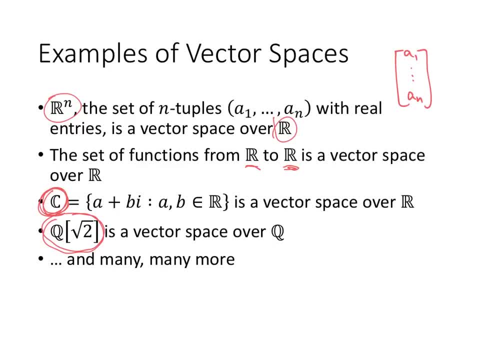 vector space. we completely ignore that And, again, there's many, many, many examples of vector spaces. Talking about vector spaces and their properties and the things that we can do with vector spaces leads to a discussion of basis and dimension and all sorts of other things that 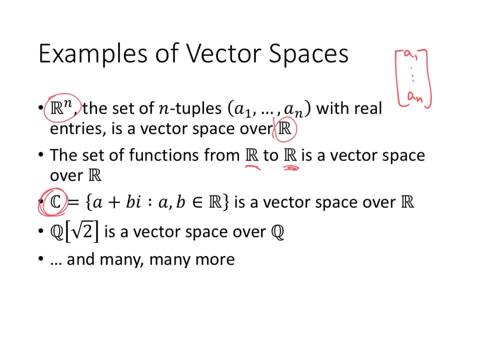 right? So this set c, if I think of it as a vector space, I'm ignoring some of the operations that can be done on complex numbers. So when we think of a vector space, we think of adding two vectors together. We think of a set of real numbers, and we think of a set of complex numbers. So when we 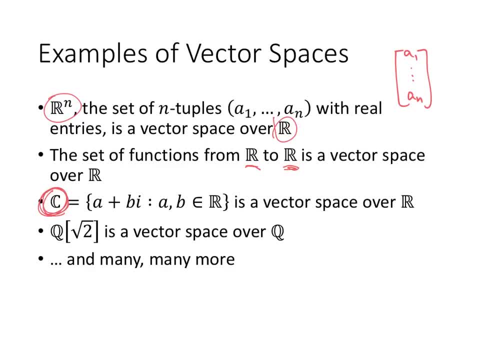 think of a vector space, we think of multiplying a vector by a scalar. But if my vectors are complex numbers, it's actually possible to multiply two complex numbers. And that operation also has a bunch of cool properties. But if I'm thinking of it as a vector space, I'm ignoring that operation that I can do of multiplying two vectors together. So in a vector space, if you have the ability to 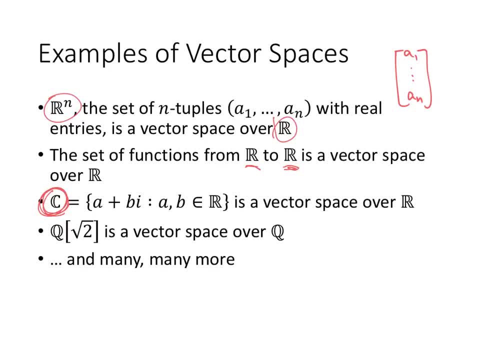 multiply two vectors together, you just ignore that. You pay no attention to that. Another example that's kind of like the complex numbers is this thing q 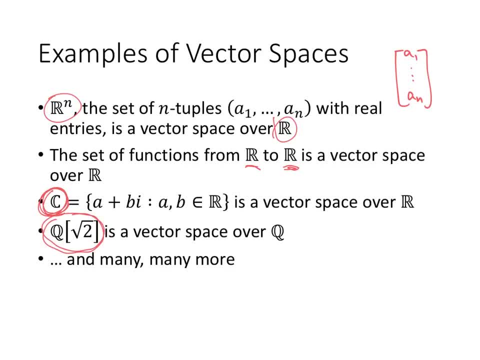 square root of two that we were talking about. Again, I have the ability to multiply two of those vectors together. But when we think of it as a vector space, we completely ignore that. And again, there's many, many, many examples of vector spaces. Talking about vector spaces and their 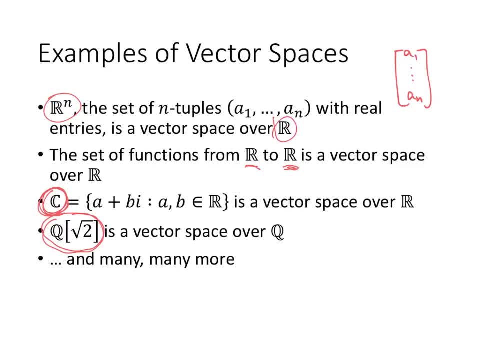 properties and the things that we can do with vector spaces leads to a discussion of basis and dimension and all sorts of other things that you might talk about in a linear algebra class. 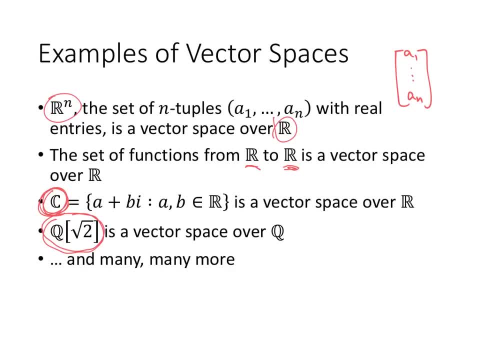 And again, that's not the focus of this video, but it's certainly something that we could talk about in another video. 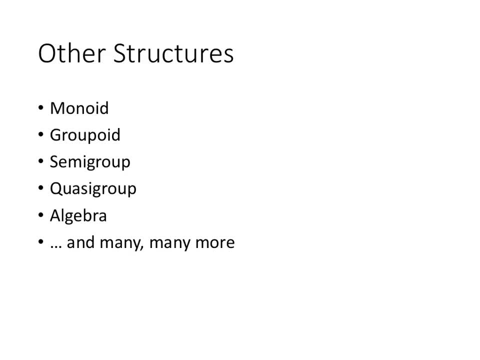 And this really is the essence of what algebra is. So when you tell somebody you're studying algebra, and what you really mean is that you're studying abstract algebra, it's easy for a lay person to get confused. You know, most people think of algebra as 2x plus 5 equals 0, solve for x. But that's not what algebra is. It's just that you're studying abstract algebra. And so when you talk about algebra, modern algebra, abstract algebra, that's not what that really represents. That represents this sort of really high-minded, you know, let's try to find common features of all of these different numerical and algebraic systems that we think about. Polynomials, matrices, numbers, all of these different things. What are some common features that we can find? That's what algebra is all about.